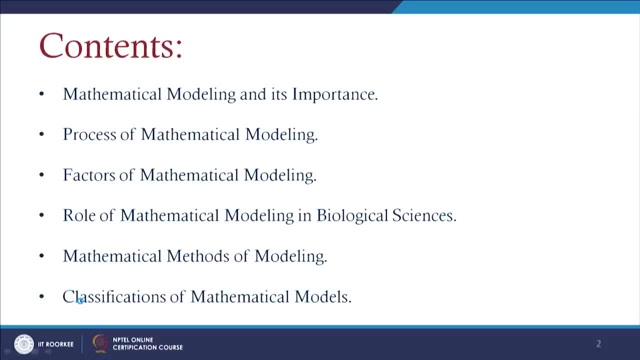 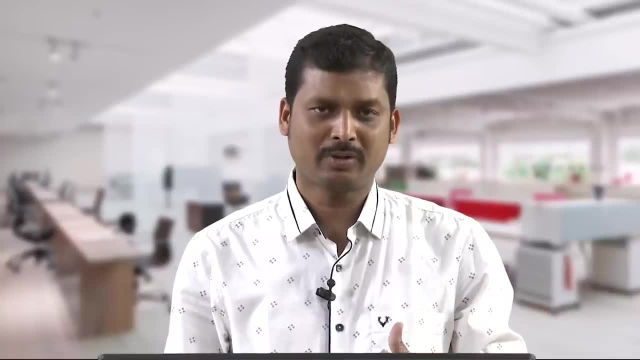 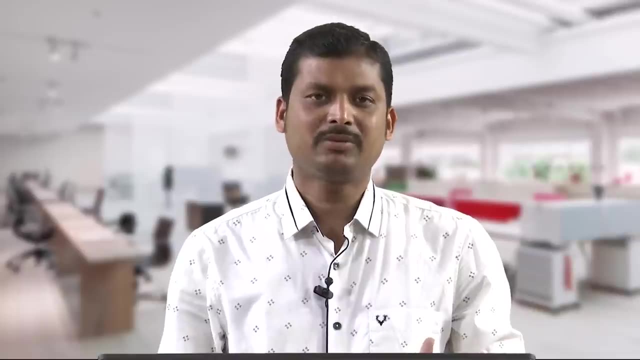 And then we will just go for this mathematical model, a development of mathematical model and based on its classifications. especially, this classification may include, like when we are just going for the mathematical modeling in biology, mathematical modeling in sociology, mathematical modeling in economics, so different class of mathematical. 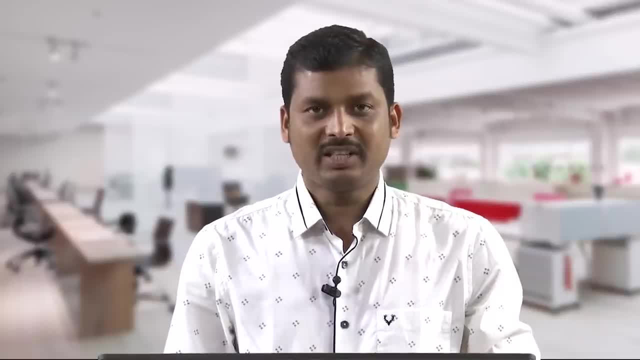 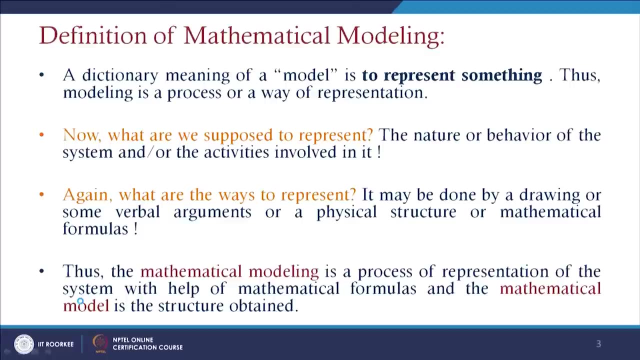 models, how we can just develop. So if you will just go for this basic definition of mathematical modeling, so the abstract model that we can just find by considering a different behavior of the system, considering a mathematical relationship, that is especially called a mathematical model. 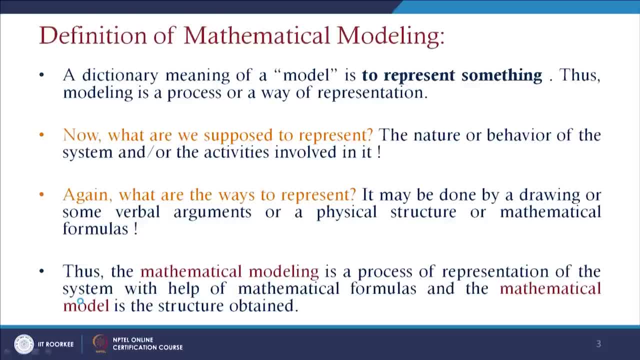 So this model means it is just to represent something. thus modeling it is a process or a way of representation of any system. So system means the collection of entities, especially called as a system. Now, since we are just representing here The nature or behavior of the system or the activities involving in it, then if we supposed 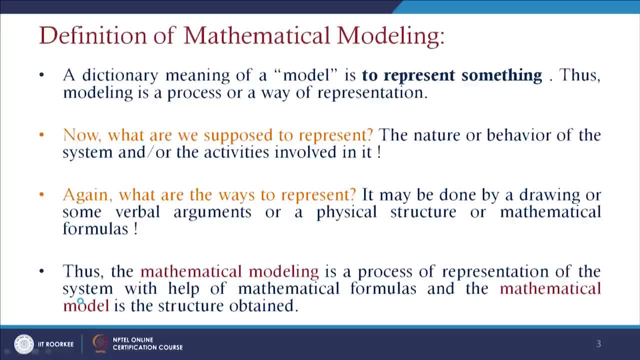 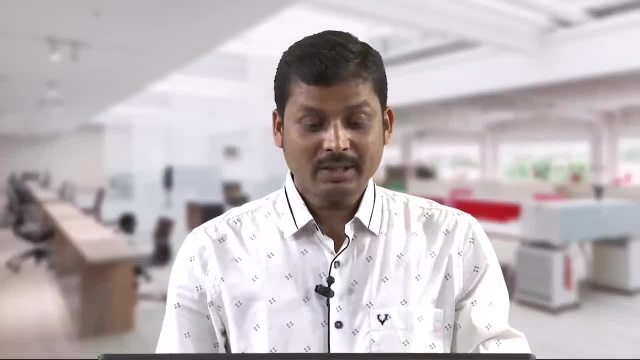 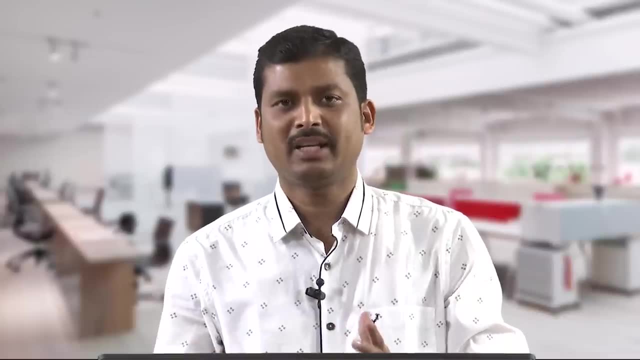 to represent all this- natural systems or like natures or behaviors- in a proper form. then we can just get a mathematical model there. Again, what are the ways to represent all this, whether we are just representing in a graphical sense or in a picturized form, or in a mathematical model. 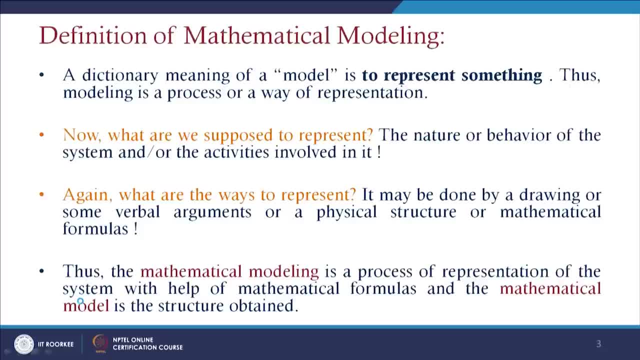 So this mathematical model, how it is differing from all other systems, especially if you will just see, You are just constructing something or you are just like representing a visual abstract, suppose. So that is especially. it is not represented in a mathematical form, but that especially. 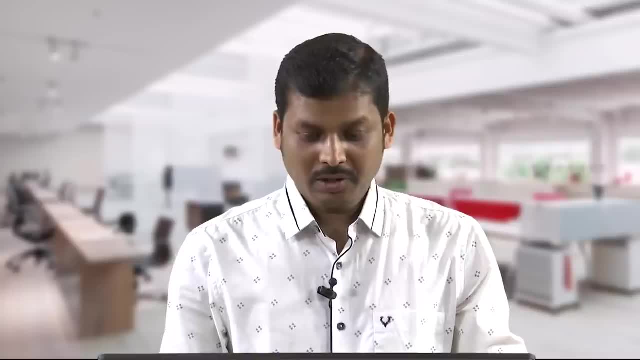 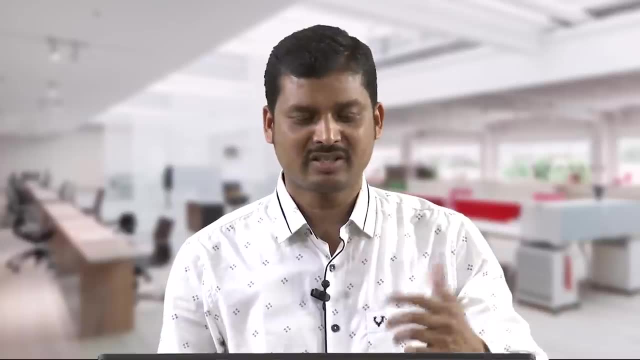 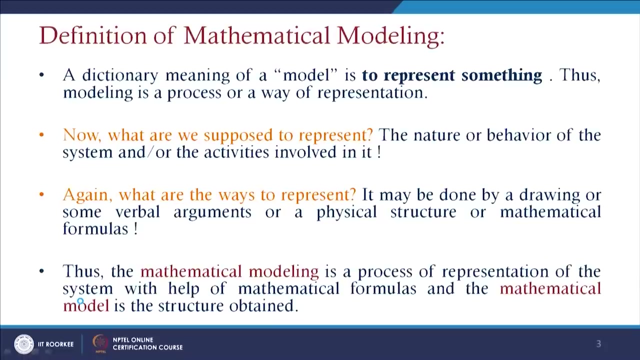 we can just say that are also models. So if it may be done by drawing some verbal arguments or physical structure or in mathematical formulas, we can just represent the systems. Thus, the mathematical model is a process of representation of the system with help of mathematical formulas. 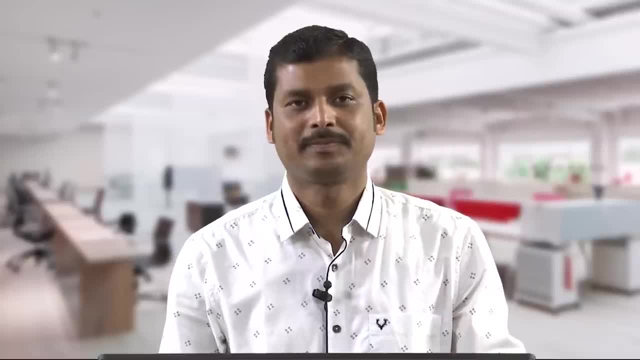 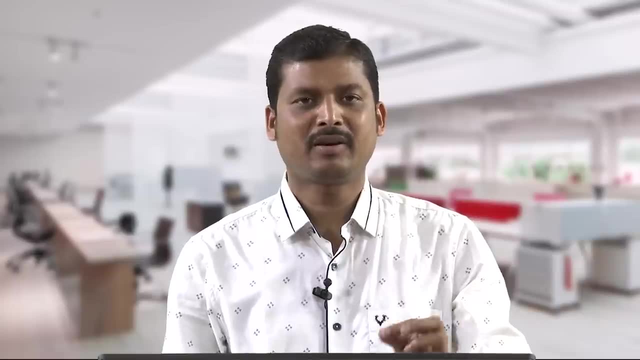 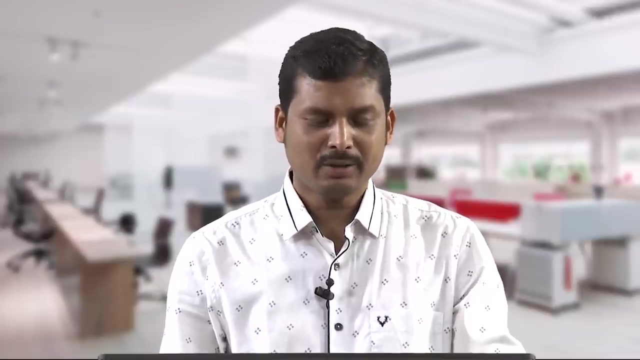 And the mathematical model is the structure to be obtained. So, especially if you will just establish this relationship with this different mathematical formulations- either it is in the form of algebra or in the form of analysis, or it is in the biological sense or ecological system sense, then we can just say: we have a mathematical. 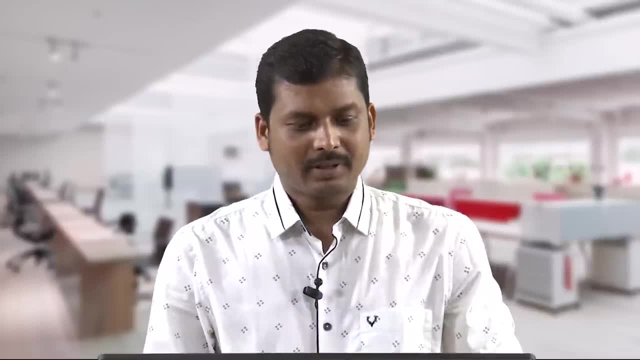 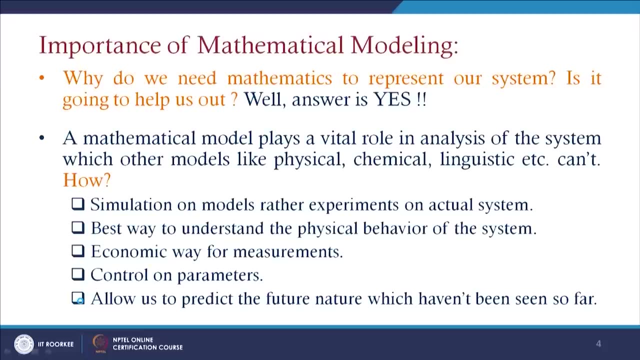 model there. So if we will just go for this importance of mathematical modeling- why we do need mathematics to represent Our system- is it going to help us out? well, the answer is yes, Since the mathematical model plays a vital role in analysis of the system. which other 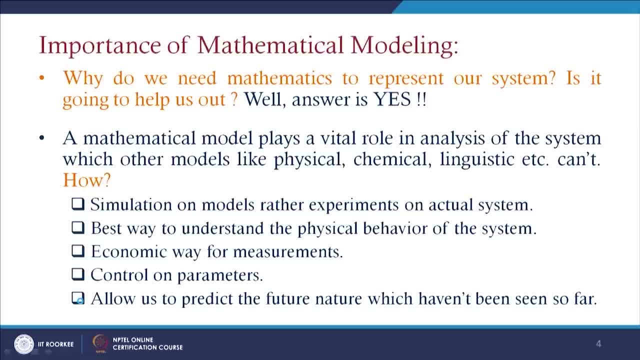 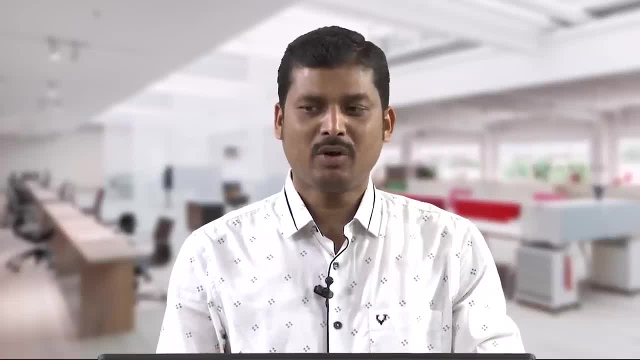 models like physical, chemical, linguistic, etcetera. it cannot do, Since if you will have a like a system, then the system can be divided into two types. one you can just say it is a abstract model, another one it is like a real experimental model. So in the abstract model, 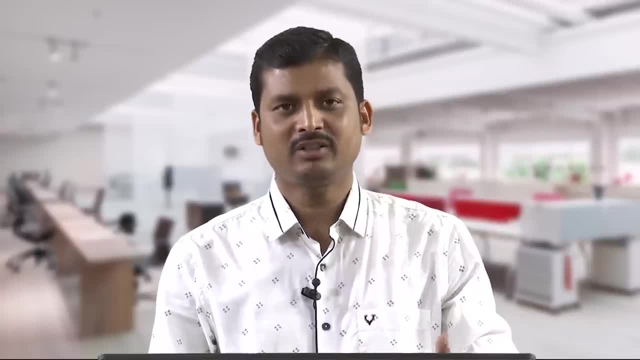 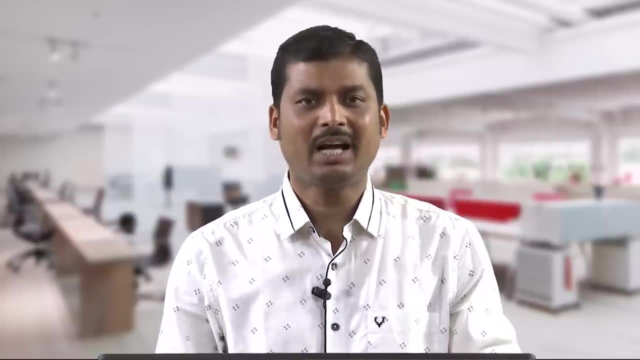 We can just Simulate or we can just try to find the solution in two forms. either we can have a like physical model, another one we can just say it is a mathematical model. and if we will have a mathematical model, then we can just find the solution of the system in two forms. 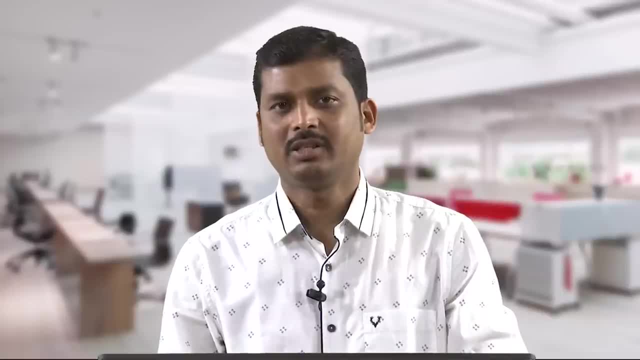 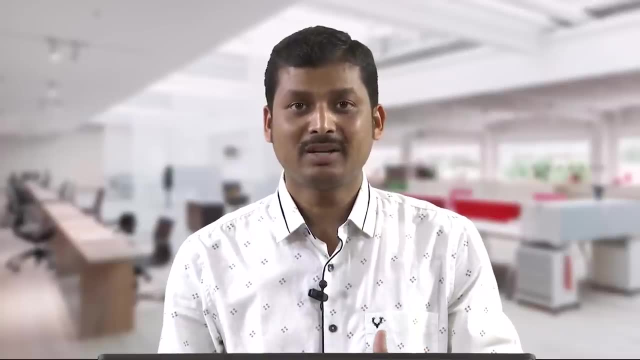 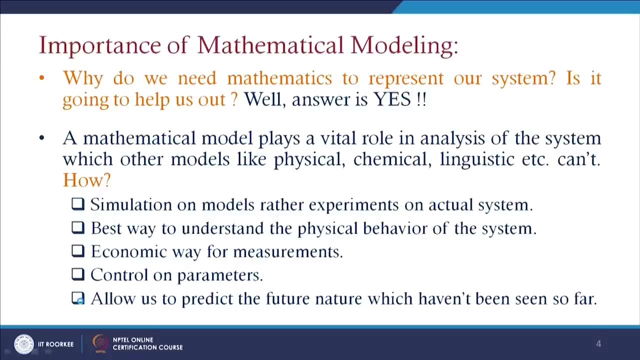 So that is either a analytical solution or a simulated result. If we will have a simulated result, then we can just compare the simulated result with the actual system, whether the system is preserving the actual behavior or nature of the system or not. So if a mathematical model plays a vital role in the analysis of the system, like suppose, 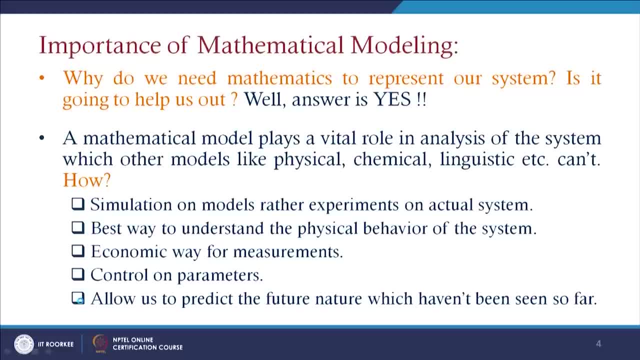 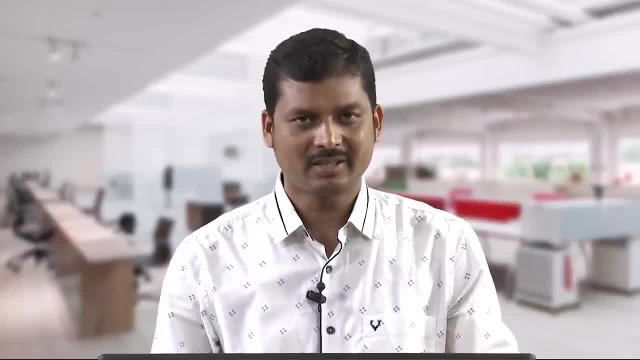 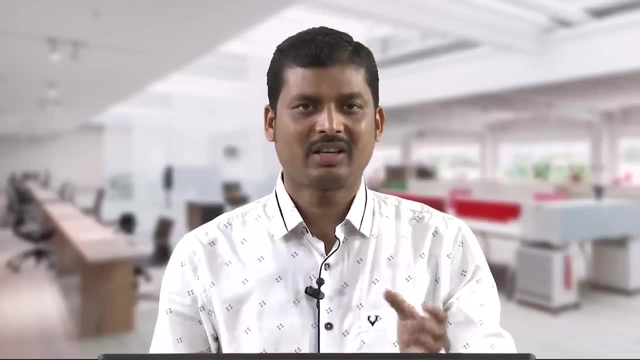 physical, chemical or linguistic systems which cannot do, then how we can do that one. So, especially if we will just do the simulation on models, rather experiments on actual system, since already I have told you that system is divided into two types. one, it is called like physical or the experimental system. another one is like a abstract model or a model which 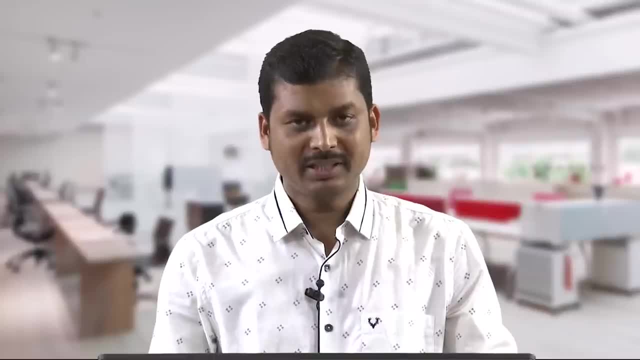 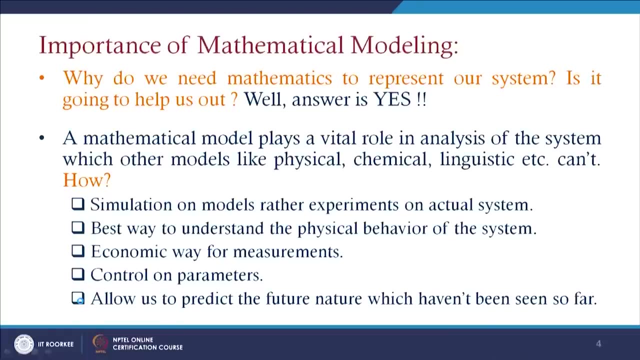 can be just constructed. So if this models can be constructed, so then we can just try to understand the actual or the physical behavior of the system in a concrete sense. So sometimes it is necessary to find the economic way for the measurements or control on parameters. 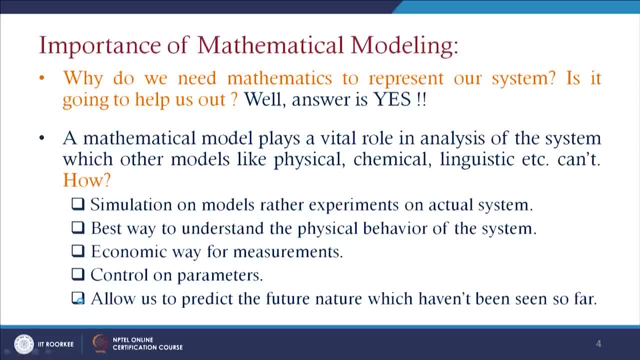 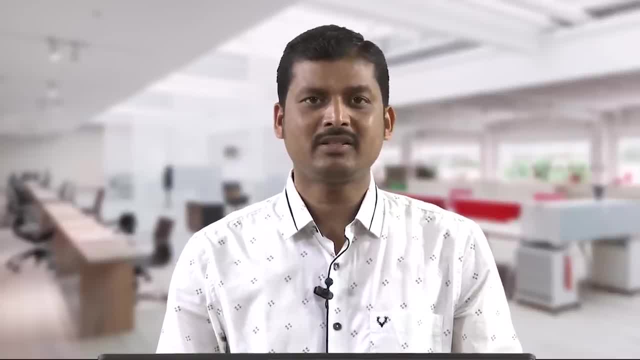 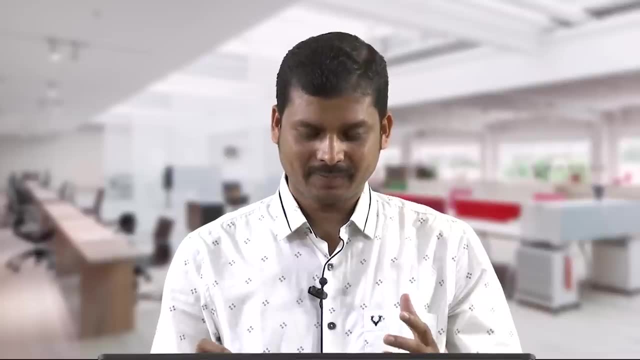 or allow us to predict that future nature which have not seen so far. Suppose, if you will just go for a like a population level, so the total population size it depends on, like the birth rate and death rate at that time level. So if you will just construct like the mathematical model based on this population, birth rate. 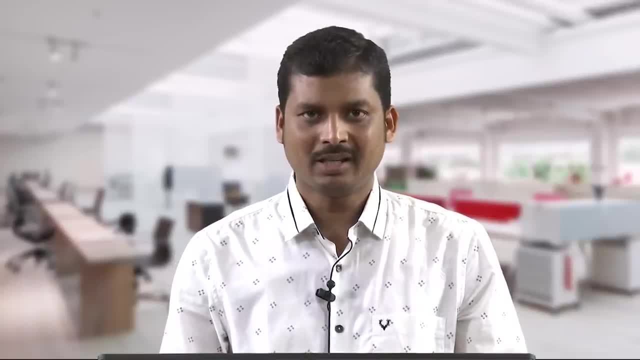 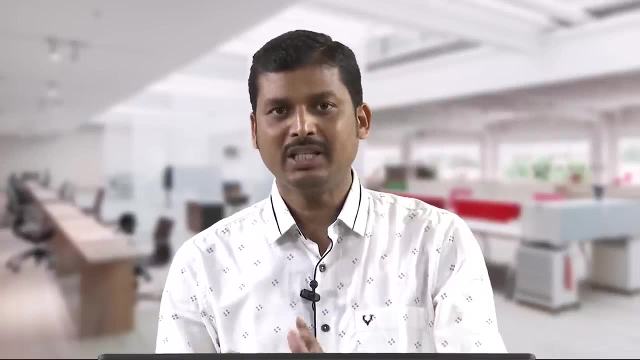 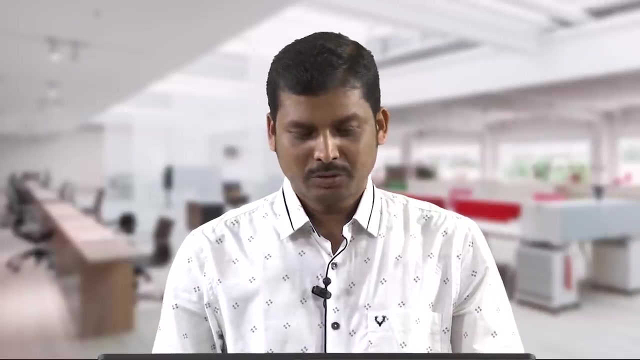 or death rate, which is proportional to the total population size. So we have to consider the past data to verify the model and based on that past data we can just say that how the future model will be. So this can be predictor or it can be made through mathematical modeling only. 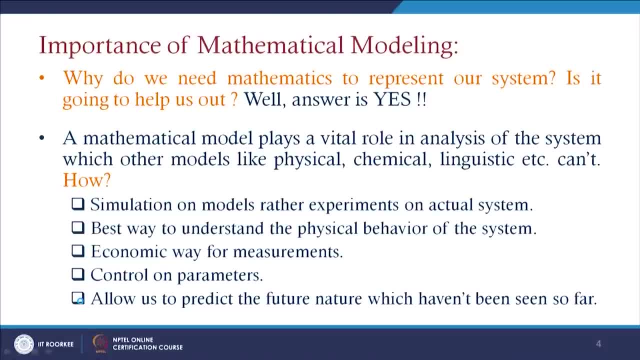 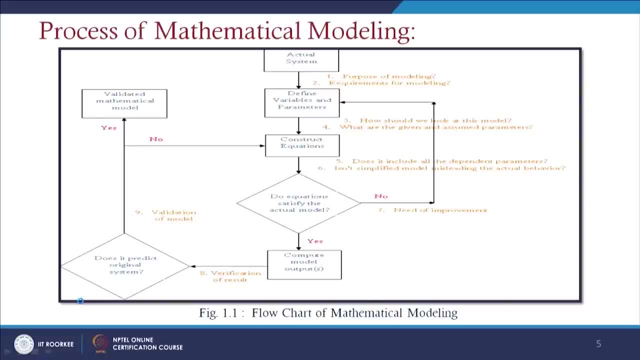 So this is our last point- that allow us to understand, Thank you, To predict future nature, which have not been seen so far. So if you will just go for this development of a mathematical model, so really we will have a actual system, then we will just define certain variables, like either you can just 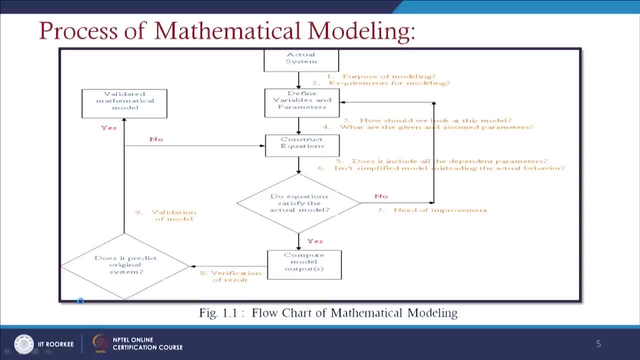 develop some mathematical relationships or you can just choose any type of parameters and then we can just establish this logical relationship with this different variables by considering certain postulates or approximations. Then we will have certain Class of equations. If this equations will satisfy or justify the accurate model, then we will go for this. 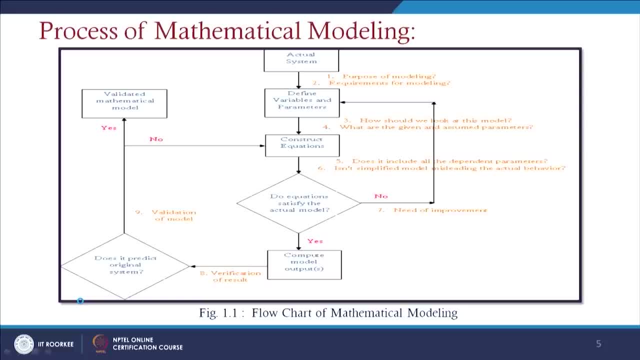 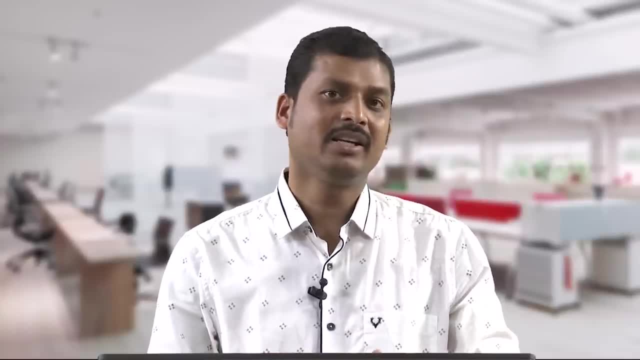 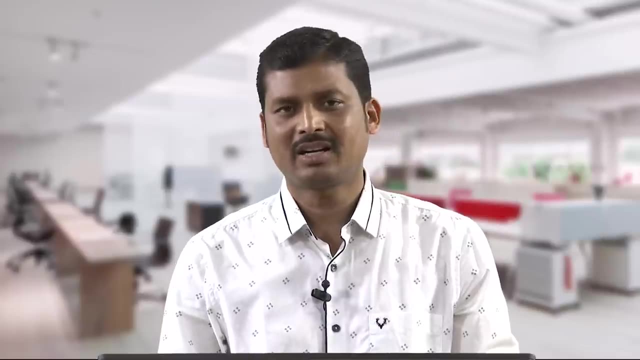 like a computational model. So if you will just compute this model data, we will have outputs here, So then that outputs can be verified with the exact system or the actual system, how it is just behaving there. So sometimes we can just collect this data. we are just plotting that one or we are just 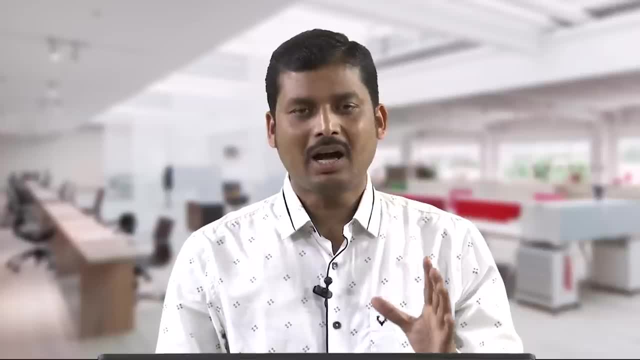 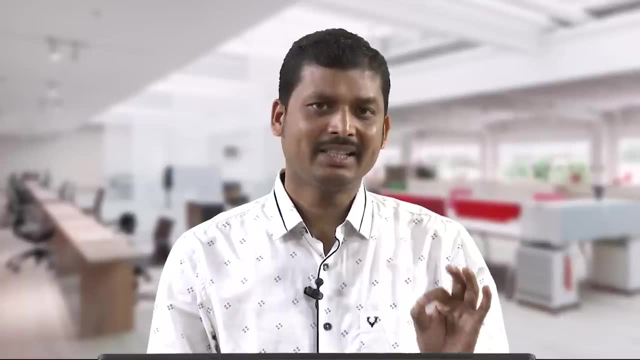 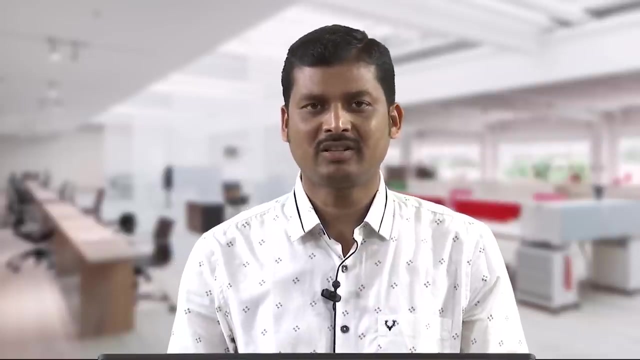 putting in different forms So to show that is the complete computed data or the like collected data or this calculated data is representing the real system in that sense or not. Suppose water is flowing. if we are just developing certain models, then we are just solving that. 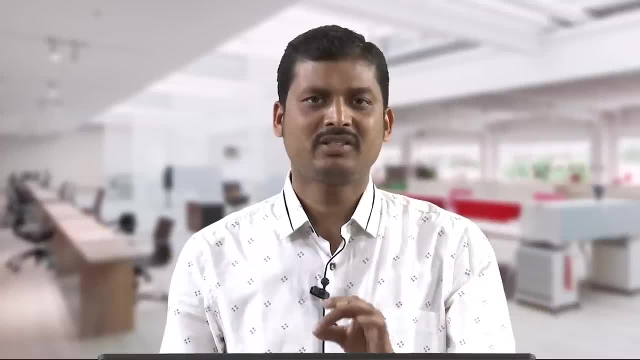 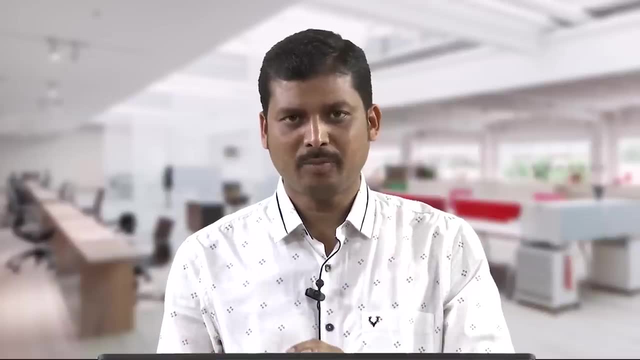 one. finally, we are just getting like certain dot points or like a certain number of a stream line points. So if you will just plot the stream line by considering, suppose, different points, then exactly It is just showing how this water is flowing there. then we can just say that like our model. 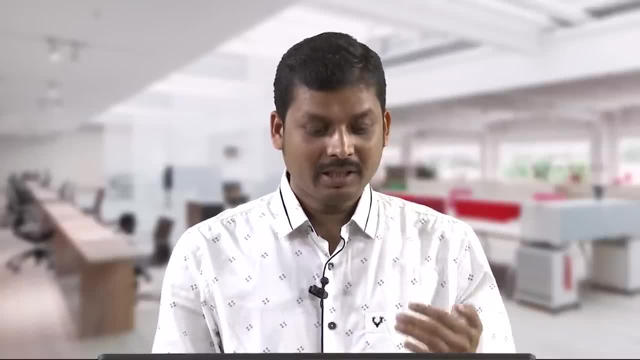 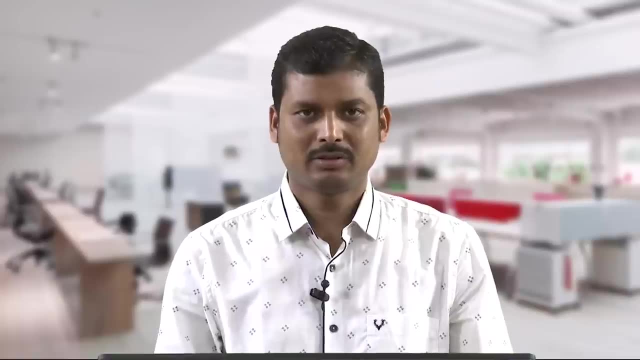 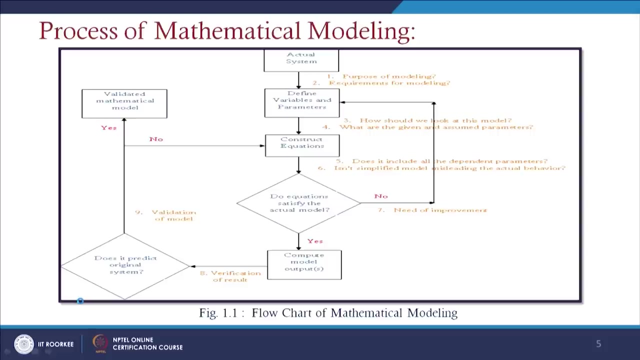 is valid in that sense. So if the verification is not proper, then we will just go for like construct of the equations again. So certain parameters we can just interchange or certain variables we can just like adjust. Then we will have different model or we will have a like new corrected model there. 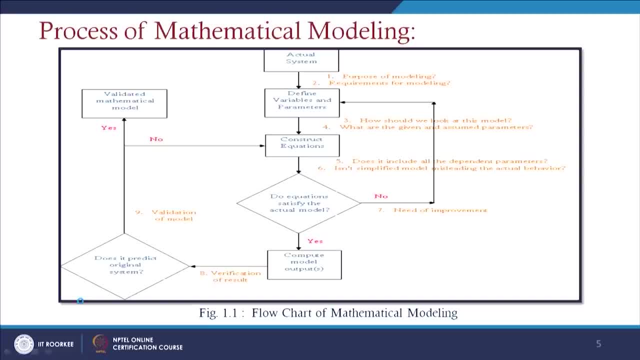 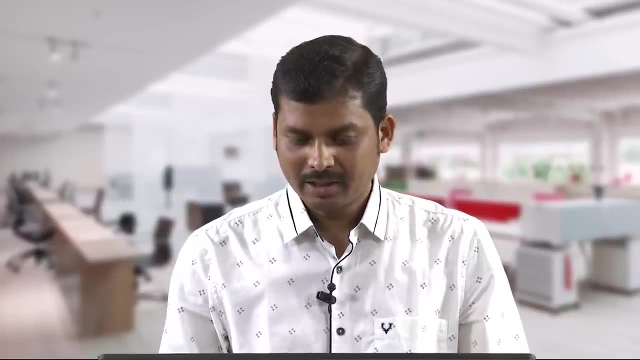 So in that model sense we can just look at At this model what are given and assumed parameters we are just using there. So if that parameters will justify the actual system in a complete form, then we can just say that all this defined parameters are correct to us. 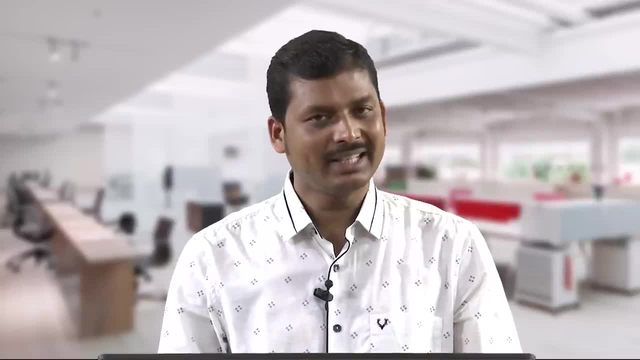 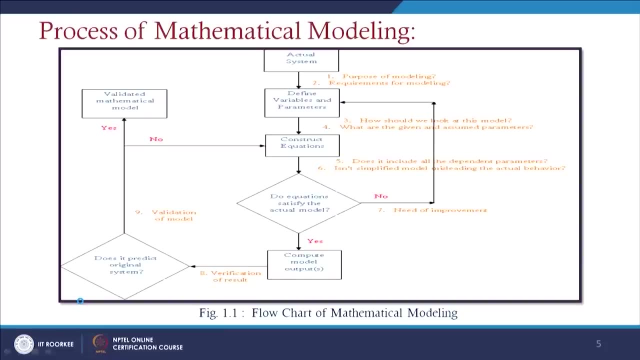 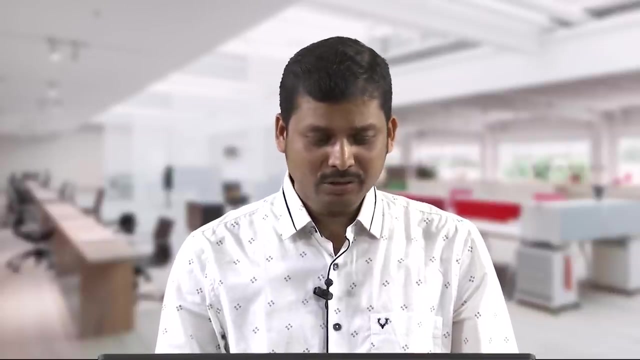 So sometimes if the simplified model misleading the actual system, then we need to improve this system in again by choosing different variables or by choosing this different assumptions, Okay, In a new level. Once it will just satisfy this complete model or the original system, then we can just say: 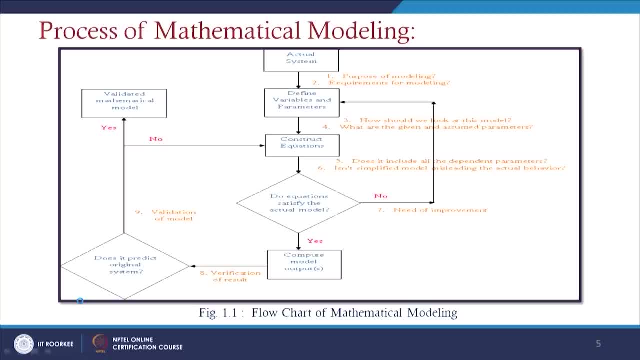 that it is a validated mathematical model, Especially if you will just see here. So we are just keeping the actual system. then this actual system takes, like this, defined variables or the parameters, And once this parameters it is just assumed, then this parameters are formulated in the 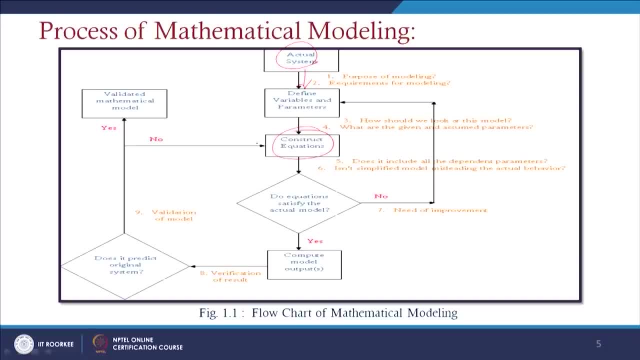 form of a Complete mathematical equations here And once we will have the set of equations, So then we can just go for the actual model there. If these equations are exactly satisfying this computed model or the defined data there, then we are just going for the verification of the result there. 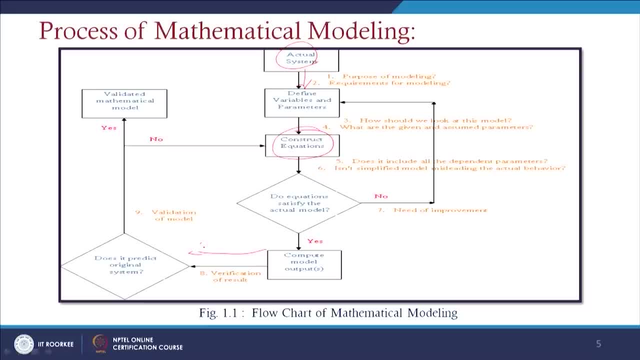 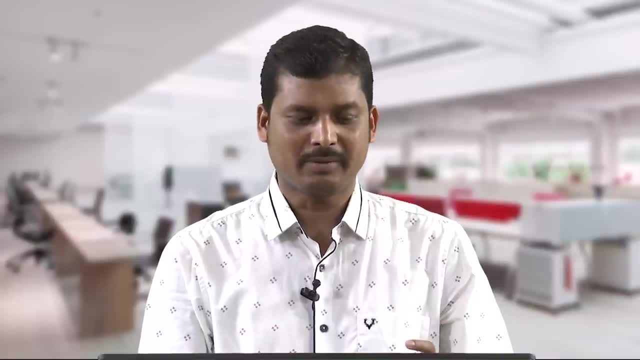 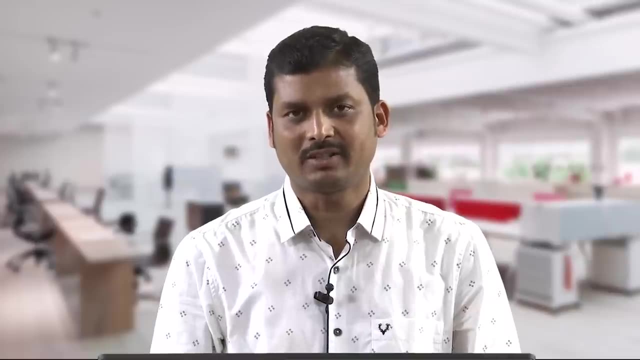 And does it predict the original system? If it is not satisfying, then we are just going again the construct of equations that by assuming or just Redefining these variables in different forms. So this flow chart is completely explaining the mathematical modeling flow chart. 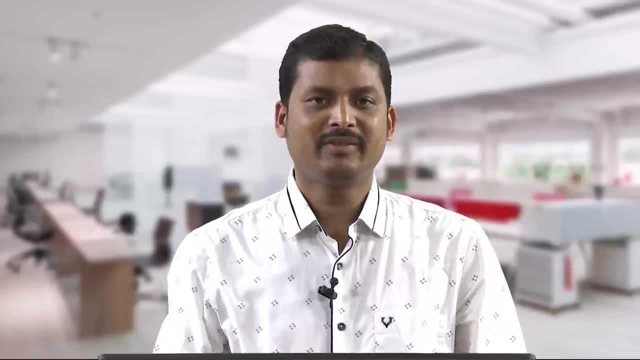 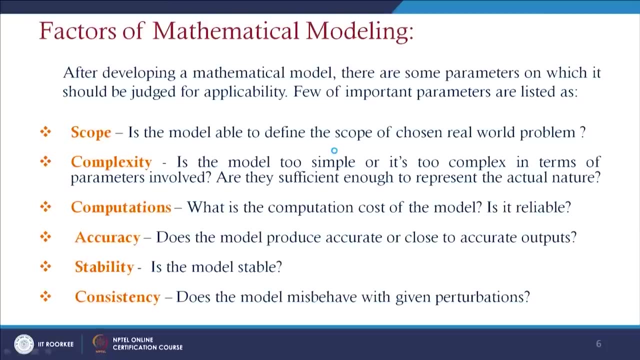 So how a mathematical model is affected by different factors that we will just discuss in this slide. So, after developing a mathematical model, there are certain parameters on which it should be judged for applicability. Few of important parameters, if you will just see. So the scope of 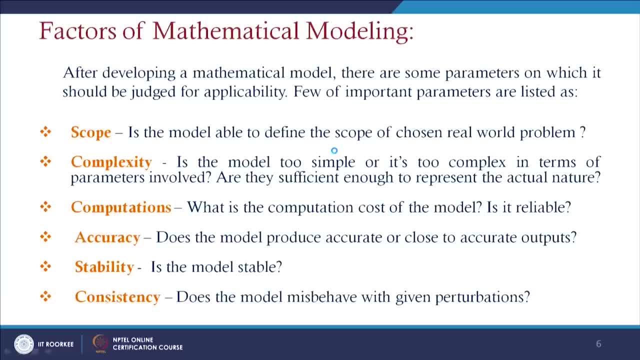 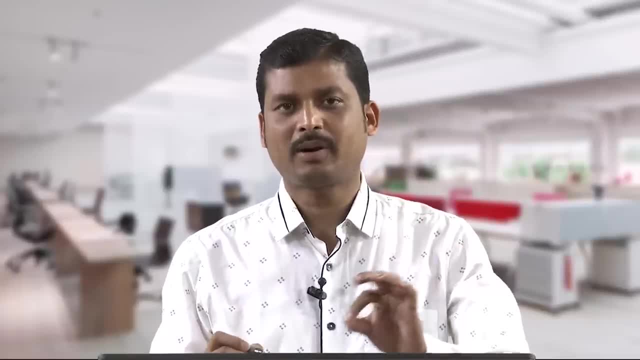 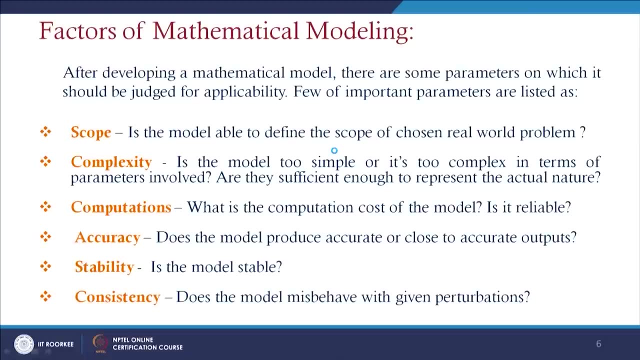 This model is: the model is able to define the scope of the chosen real world problem. So this means that once you are just developing a mathematical model, whether that fits properly with the exact system or the actual system or not, So then the complexity of the problem is: the model is too simple or it is too complex, since 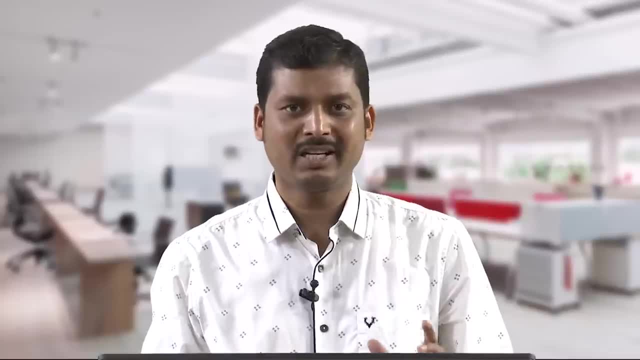 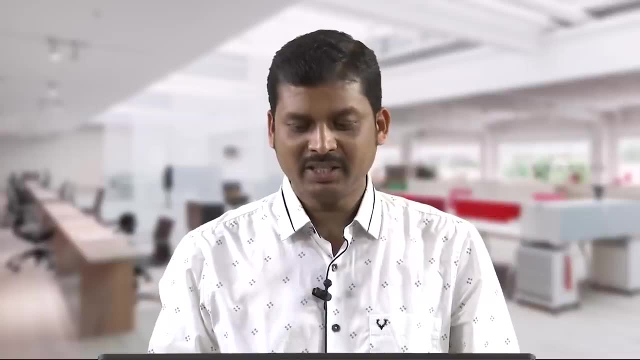 if it is a complex mathematical model or a complex equations are involved, it is difficult to find the solution also sometimes Since lots of parameters it will be get involved And it is difficult to find the solution also sometimes And it is not sufficient enough to represent the actual nature. 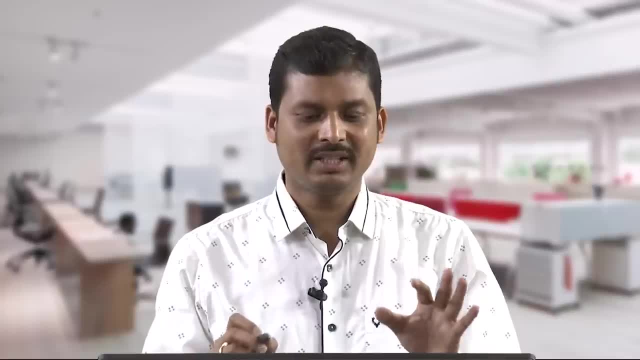 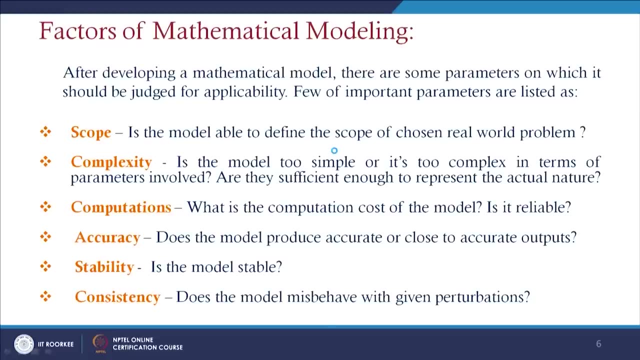 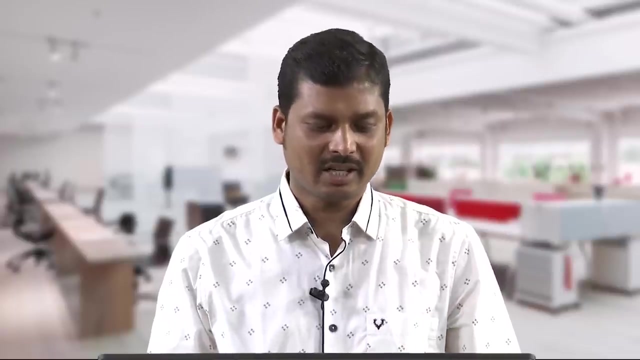 So then, if we are just formulating this model, whether it is simple or complex, then we will just go for the computations. What is the computation cost of this model, Since sometimes maybe this model will take like one day computation, or sometimes it may require a huge amount of devices to get the result there of? 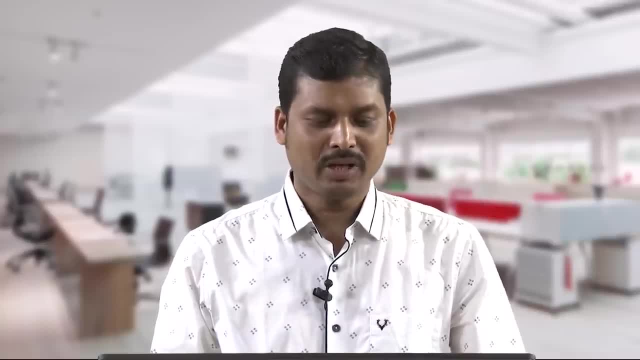 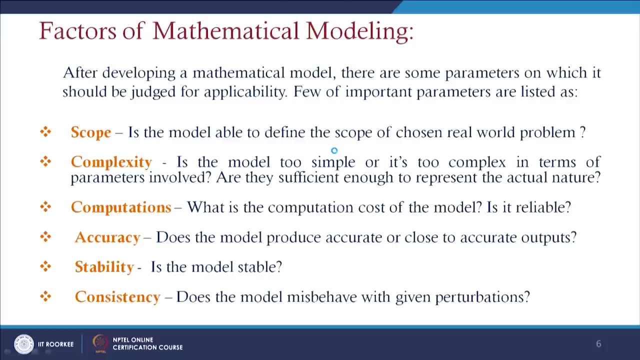 So that we have to keep it in mind that when we will just go for a simplified model or a complex model, So once this result is just get it out, then whether this model produce an accurate or close to a solution which should be produced by the actual system or not, that we have to. 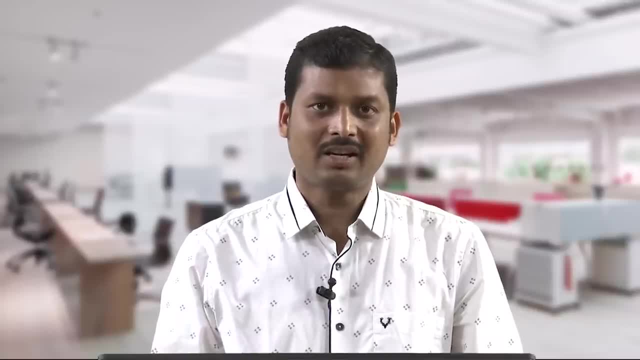 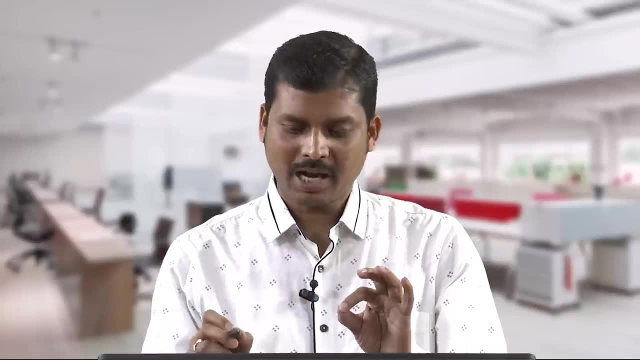 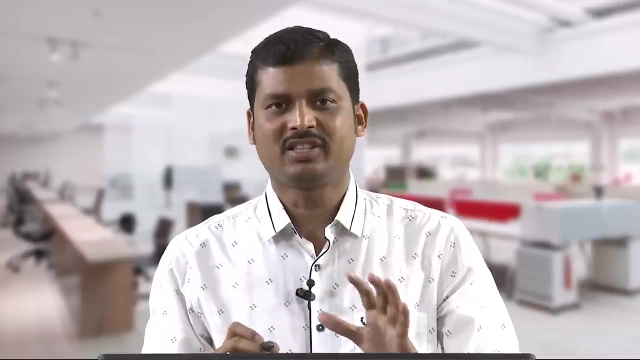 see also, Sometimes the systems are just destabilized itself. This means that if we are just going towards the actual model, then it will not go towards the exact solution there. It will just deform from the actual system. Then we will have like instability condition. 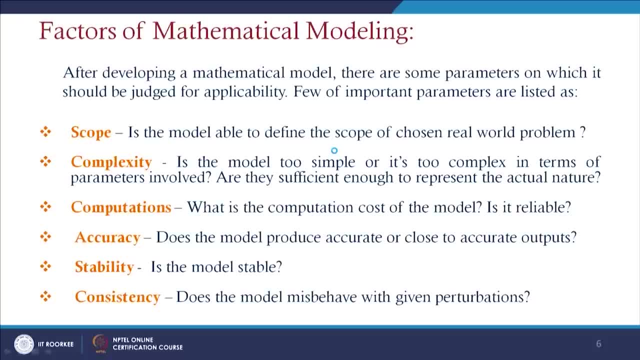 So we have to go for the stability of this model, That how the stable condition or how this parameters. if we are just defining in the system So it should provide a stable solution to us, Then we will just go for the consistency. If the system is not consistent, then we will not have a feasible solution. 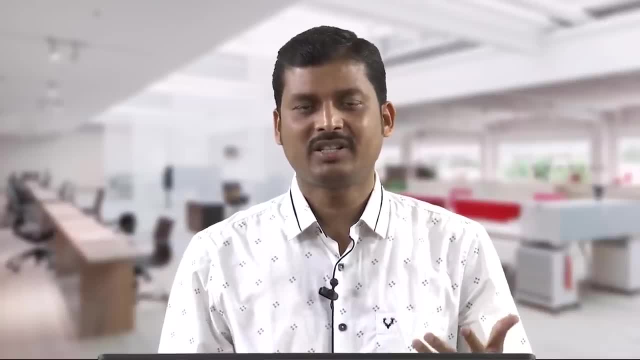 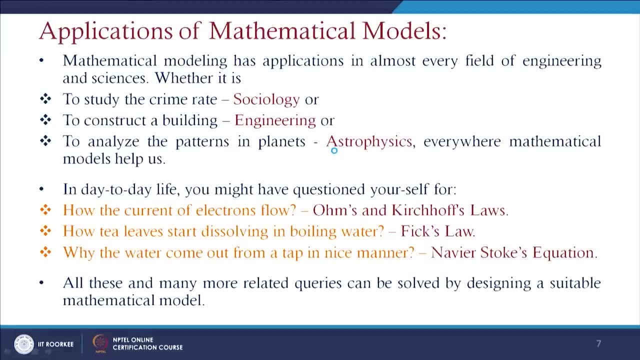 So if we don't have a feasible solution, then we cannot say that our system is a fully equipped with this mathematical model. Thank you. So then we will just go for the applications of mathematical model. Sometimes, if the real system, if we are just doing the experiments, many times it is not. 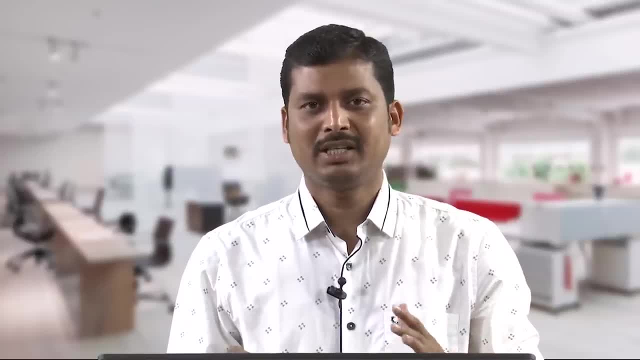 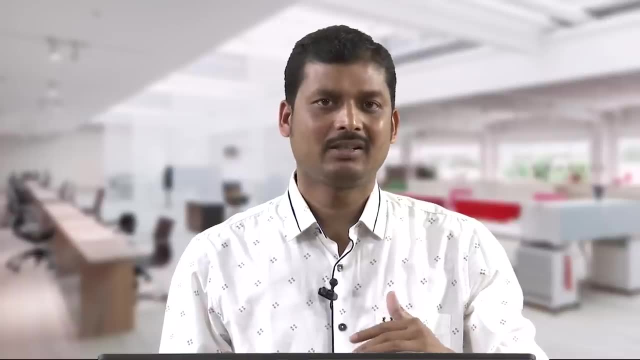 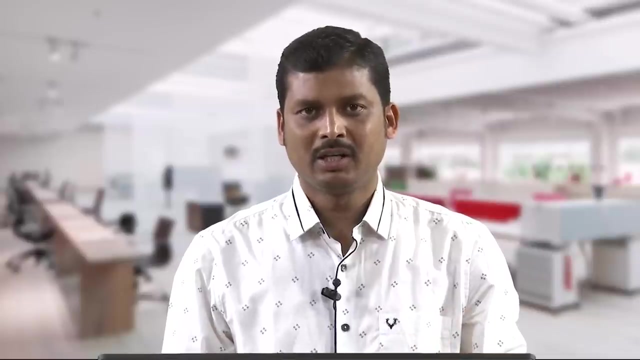 possible to do or to conduct the experiments in actual sense also If, suppose in a, like a paper mill, suppose if the temperature is go beyond, like, go above, like a 1000 degree Kelvin. So it is not easy to handle. if there are small, accidents are going on. 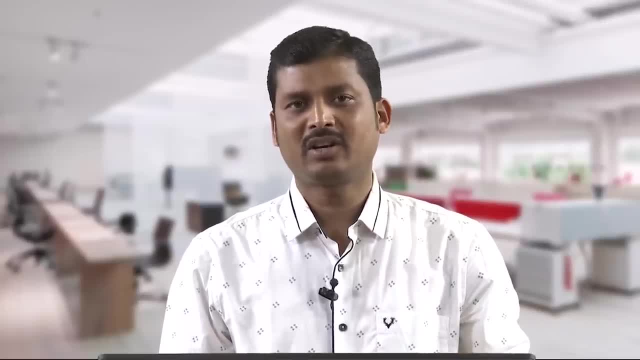 So especially what people are doing is they are just formulating a mathematical model. So it is not easy to handle if there are small accidents are going on. So especially what people are doing is they are just formulating a mathematical model. Then they are just going for the experiments. 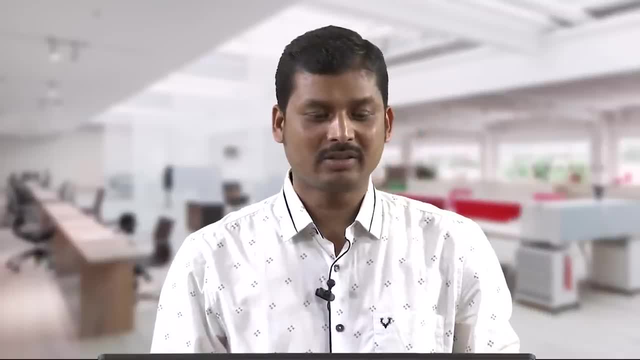 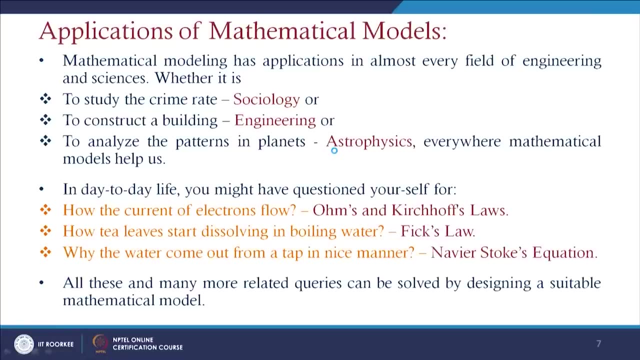 So in that sense, where we can just use this mathematical models, that will just take care. So if you just see, mathematical modeling has applications in almost every field of engineering and sciences, Whether it is in a like to control the crime rate in sociology or to construct a building. 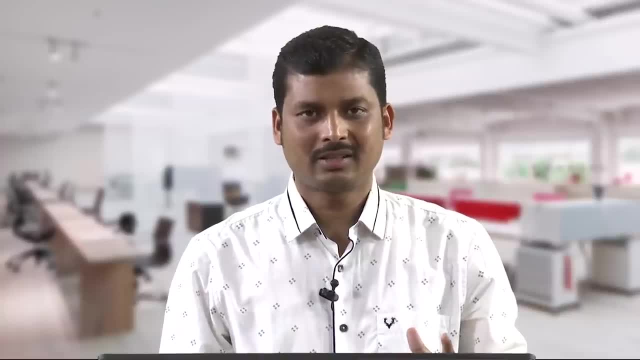 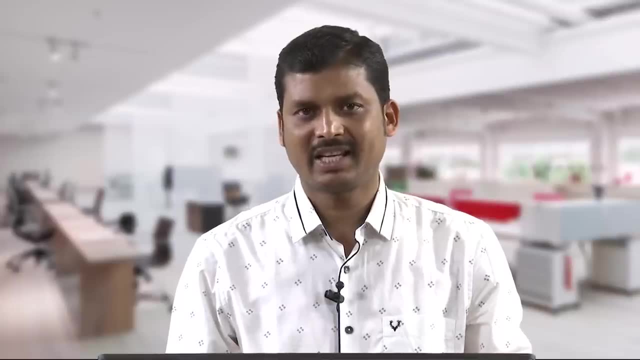 so especially. you just see fracture mechanics. It is just. you'll just see, it is not a set of equations only like stress components, are there strain components? are there different tangential factors? it is just involved, that is nothing. 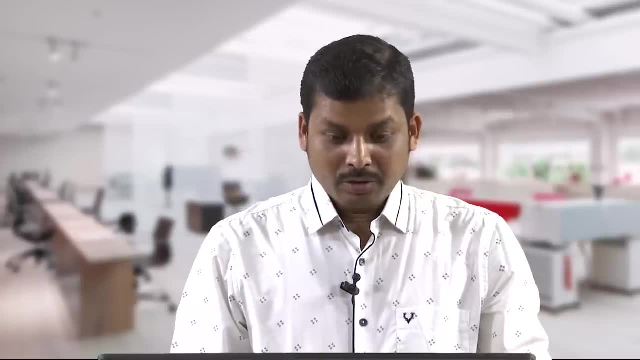 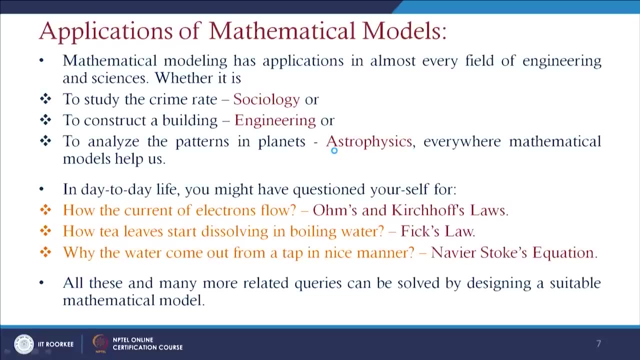 but the mathematical models only. So if you'll just go for the analyze, the patterns of planet, suppose, in astrophysics, so you can just find that there requires also a mathematical model to visualize all this like computations or like the movement of this planets in the space. 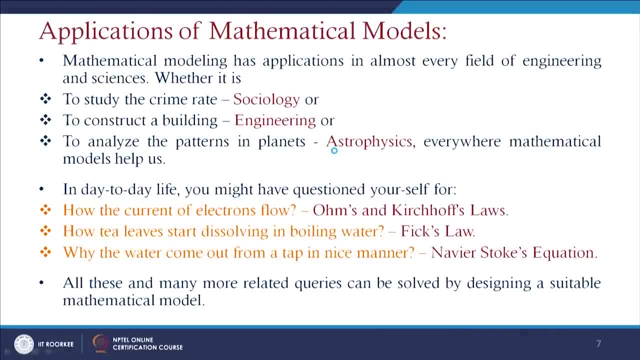 In day to day life. you might have question for yourself how the current of electrons flow, So, especially if you'll just see this, always satisfy this Ohms and Kirchhoff's laws. so that is nothing but the representation of some of this mathematical relationships. 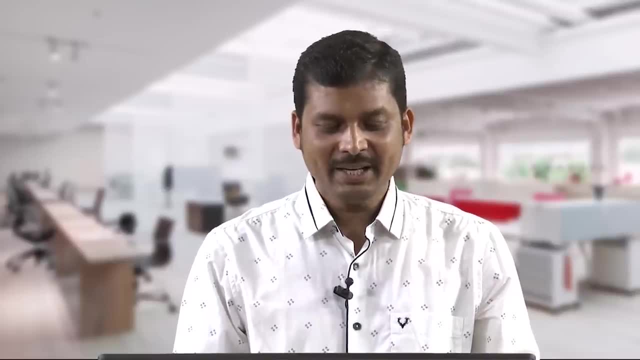 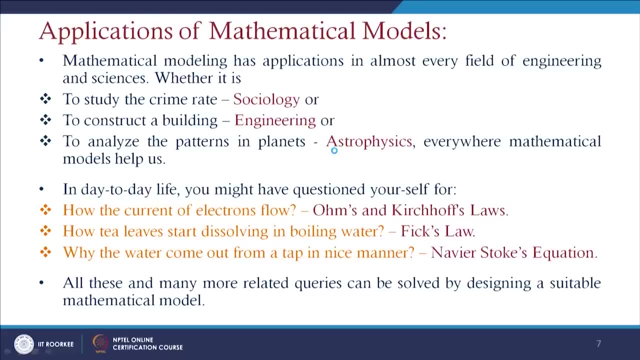 with certain number of variables. So how tea leaves start dissolving in boiling water- fixed law of diffusion- why the water dissolves Come out of the tap in a nice manner- Navier-Stokes equation. So if you'll just see Navier-Stokes equation, it involves only the partial differential. 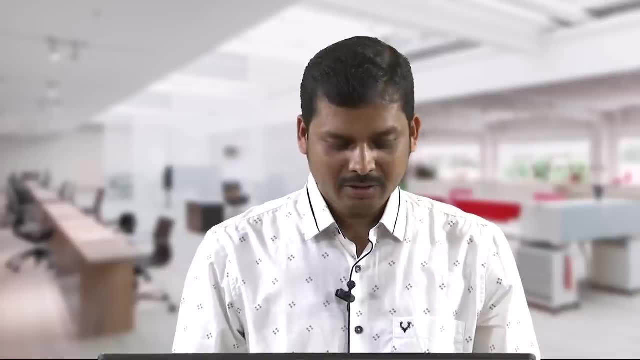 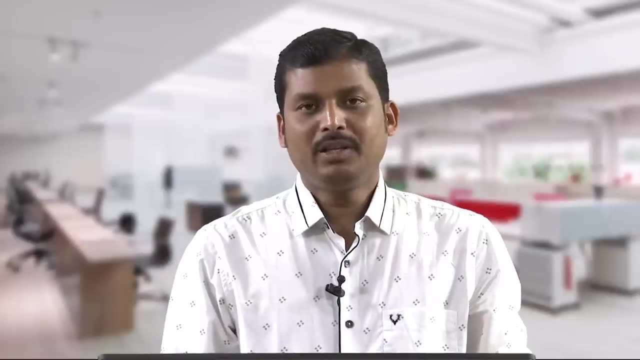 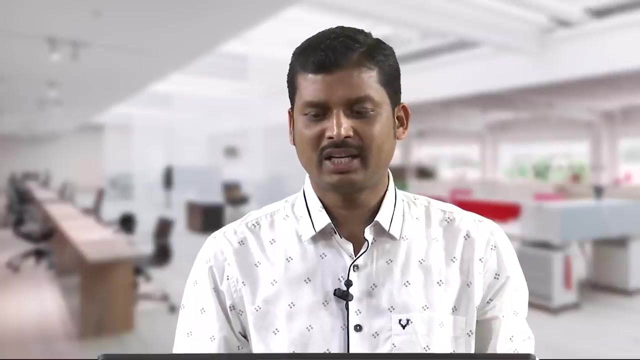 equation with certain non-linear terms are present. So all these are many more related queries can be solved by designing a suitable mathematical model. So if you'll just go for this scope of mathematical modeling in a ecological sense or in population balance modeling or in biological sciences, you might be amazed by looking at nature's 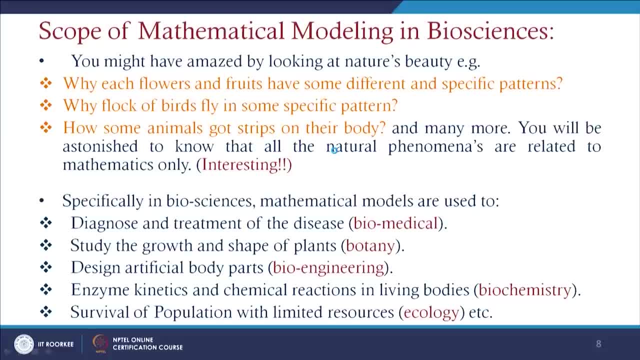 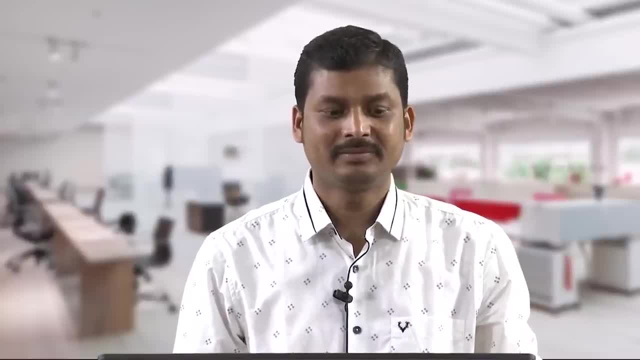 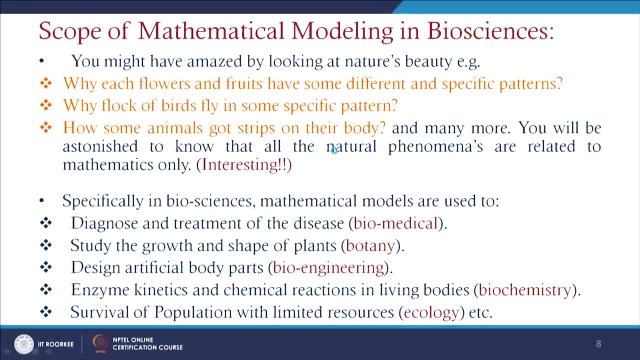 beauty also sometimes Why each flowers and fruits have some different and specific patterns. You can just find that it follows a mathematical relationship there, Why flock of birds fly in some specific pattern, How some animals got strips on their body, So always you can just find there establishes a relationship with the mathematical terms. 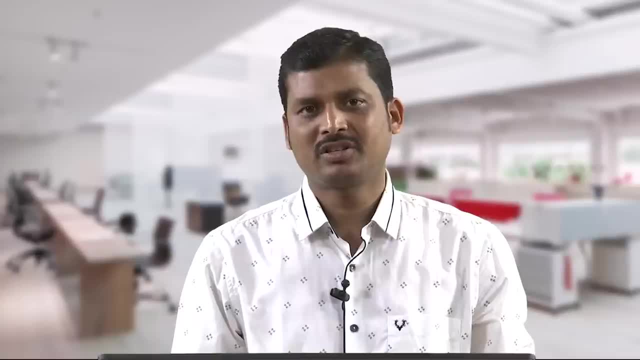 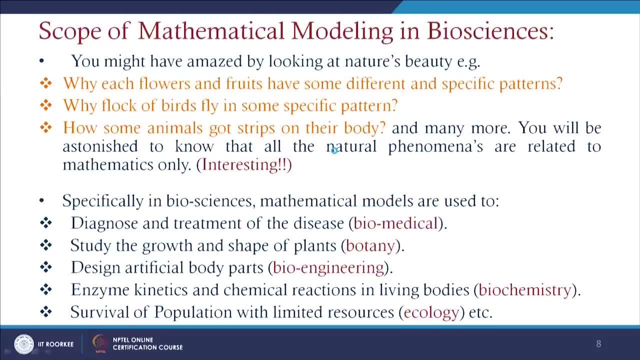 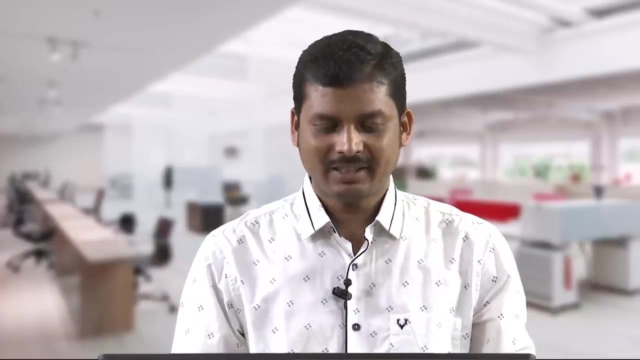 there and so many things. you can just find that everywhere the beauty of mathematics is present. You will be astonished to know that all the natural phenomena's are related to mathematics only. So this is very interesting, specifically in bio-sciences. you can just find that mathematical. 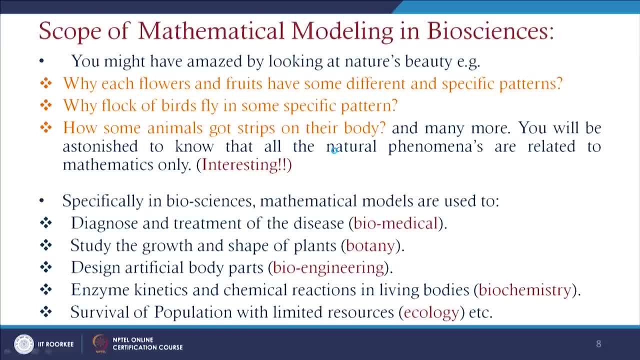 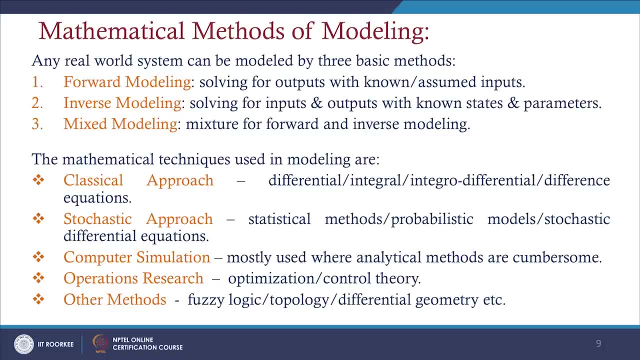 models are used to diagnose and treatment of the diseases, Study the growth and shape of plants, design artificial body plants, enzyme kinetics and chemical reactions in living bodies. then survival of population with limited resources, that is ecology. So in mathematical modeling we'll just use different mathematical methods, especially 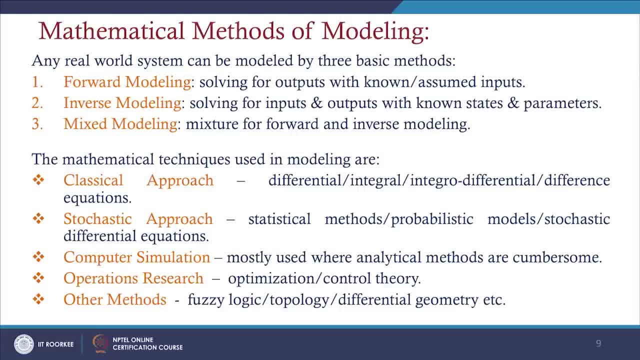 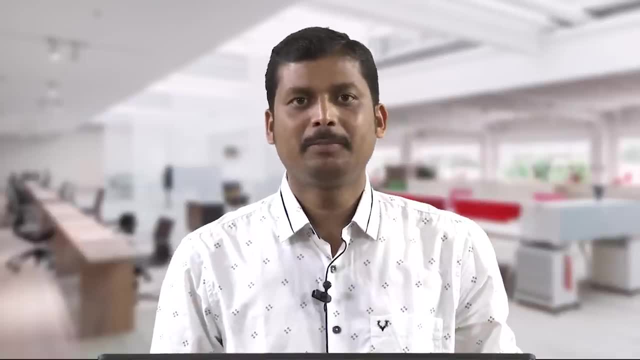 any real world problem can be modeled by three basic methods. One, it is called forward modeling, that is, we'll have like inputs and we'll just go for outputs, especially if you can just see, for example, like a triangle. So if P and B are known to you, then H it can be computed by using P and B. 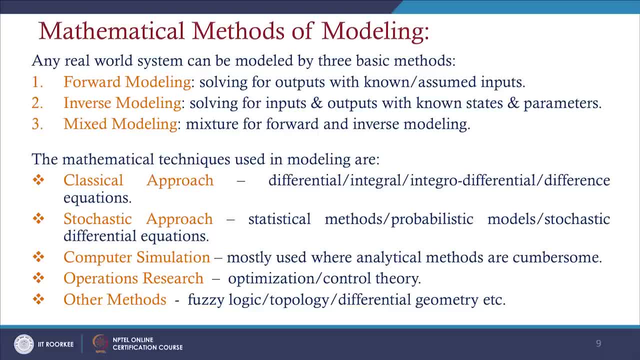 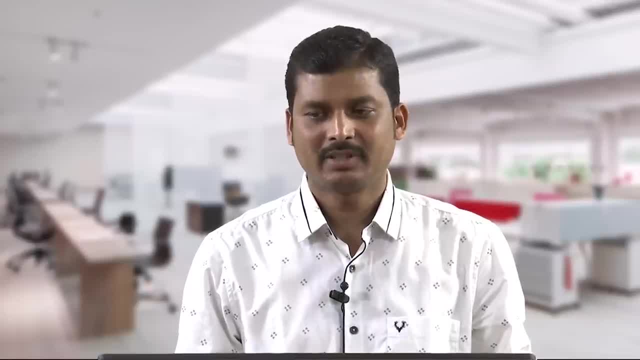 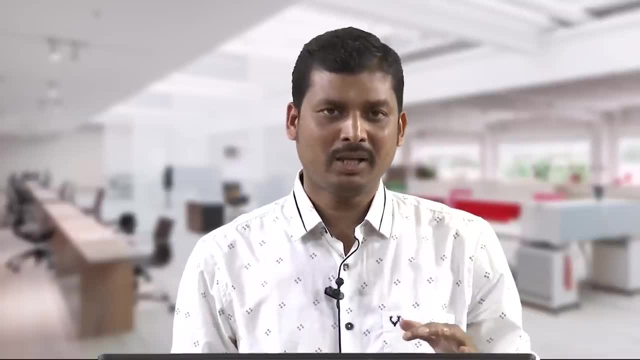 And in inverse modeling. so this means that you will have this output and you will, or you want to know the input there. especially if you'll just discuss here astrophysics, then you can find that when this solar rays are coming and when this rays are impacting, 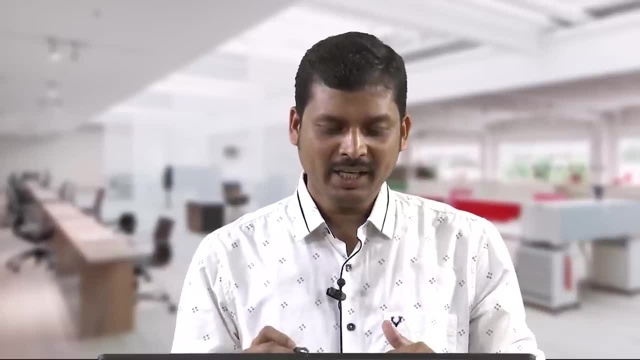 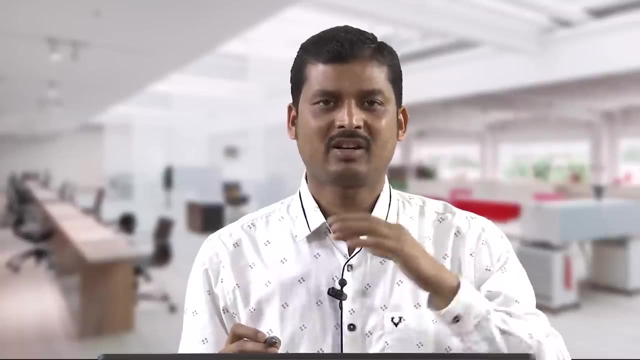 on the ground, from the ground data itself. we are just going in a back form or in inverse modeling form to find that what composition of gases or radiation effect, it is just a scattering in solar space. Then in the third we'll just go for mix modeling. 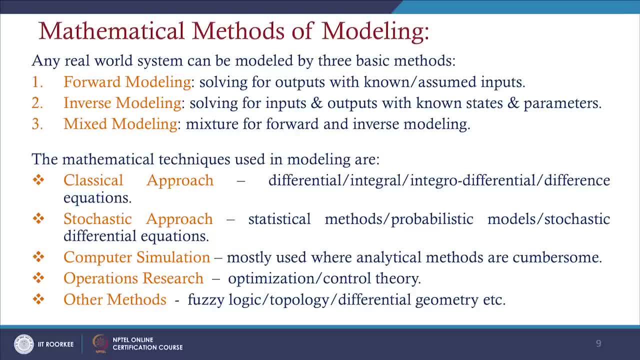 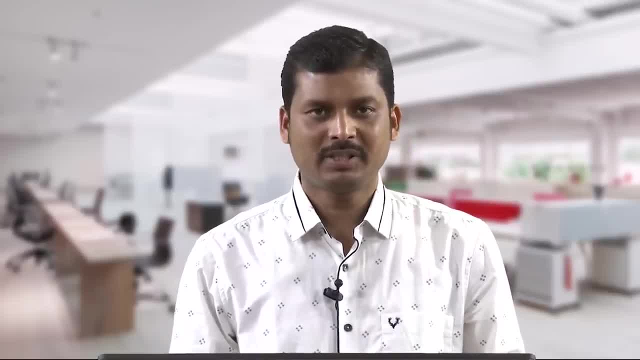 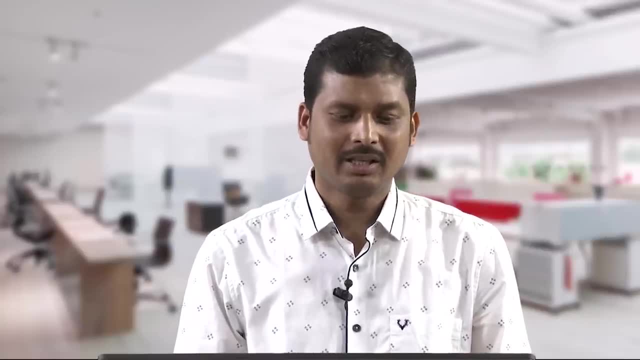 So in a biomedical imaging sense you can just find that some data they are using forward modeling sense, or some of the data it is used for inverse modeling to get the complete solution. So especially that is used for many physical scenarios. that is especially called mix modeling. 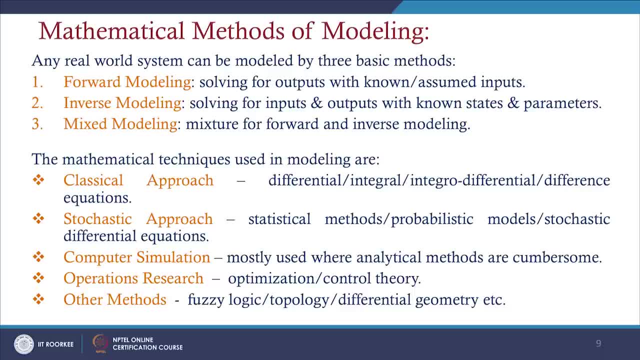 Now any system, if you'll just see we'll have, either it is in forward modeling sense or in the inverse modeling sense. So if you'll just go for this, mathematical technique is used in. the modelings are, like, defined in a five forms here that is first. one is classical approach. 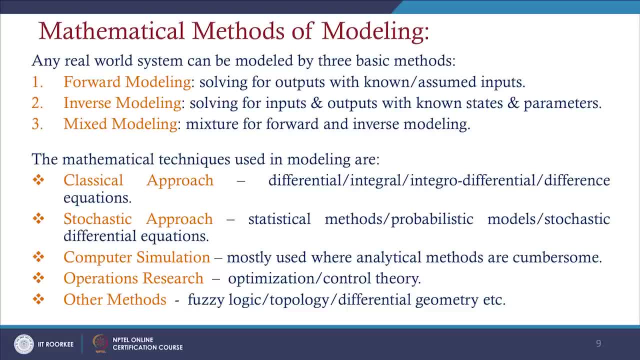 So classical approaches are used for like differential, integral, integro differential or difference equations. Second one is a stochastic approach. In the stochastic approaches we are using statistical methods, probabilistic models or stochastic differential equations. And if you'll just go for this, 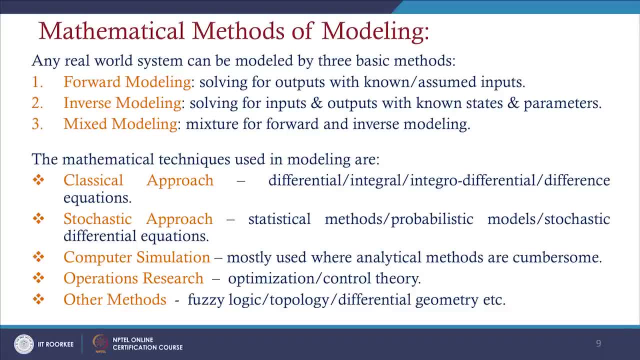 Third class of technique is, that is, computer simulation. In the computer simulation mostly we are just using analytical methods to find the exact combination of the solutions. Fourth one is operation research. So usually the optimization technique is, or control theory is used to find the solution. 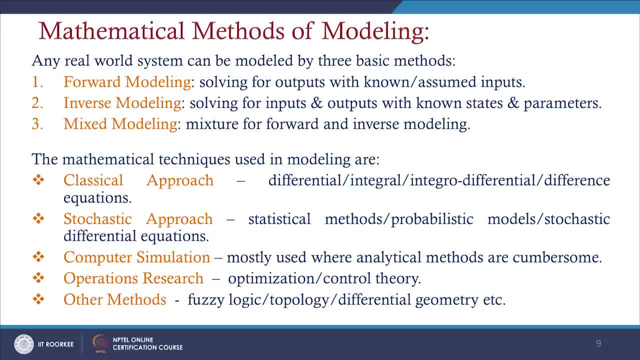 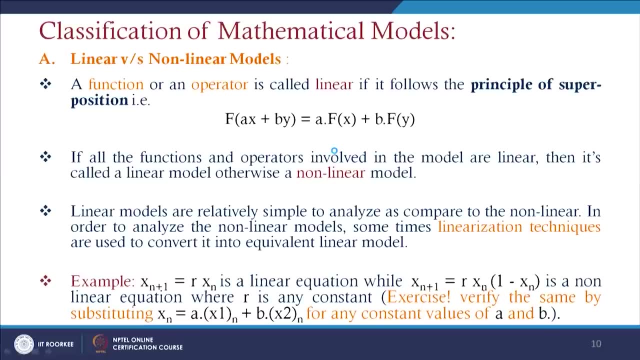 process And other methods like fuzzy logic, topology, differential geometry, etc. it is just used to find certain class of problems. So then we'll just go for this classification of mathematical model. So, especially if you'll just see, this classification depends on whether we'll have a linear system. 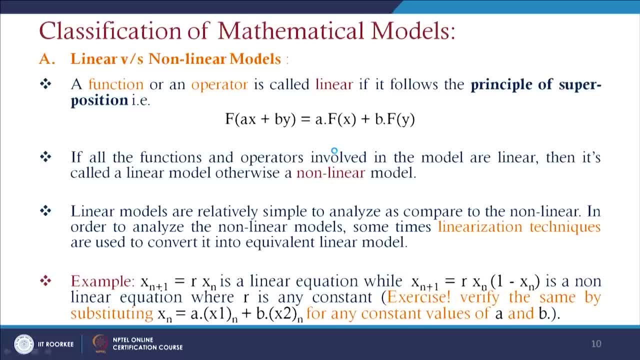 or we'll have a non-linear system, Especially if you'll have a linear system, we can just say that it is a linear model. Then, if you'll have like non-linear system, then we can just say that it is a non-linear model there. 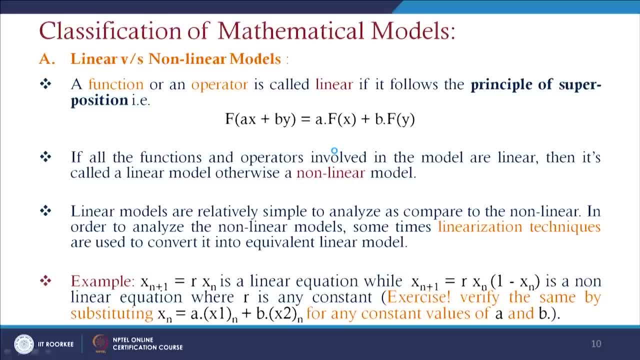 So if you'll just go for this like comparison of linear and non-linear model, we can just find that Any function, For any operator, It is said to be linear if it follows the principle of superposition. That is especially if you'll just write any function which can be defined as f of 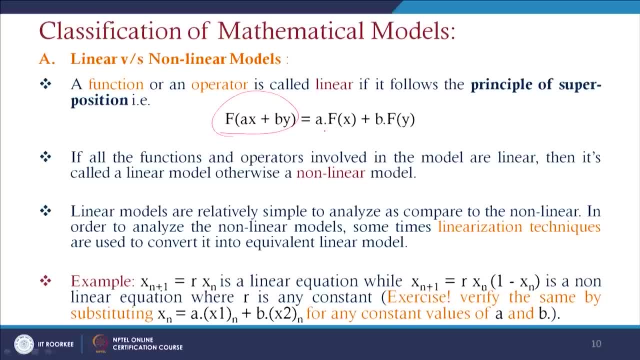 x plus by, which can be written as a into f of x plus b into f of y, where a and b are constants and x, y are the variables. then we'll have a linear operator If all the functions and operators involved in the model are linear. 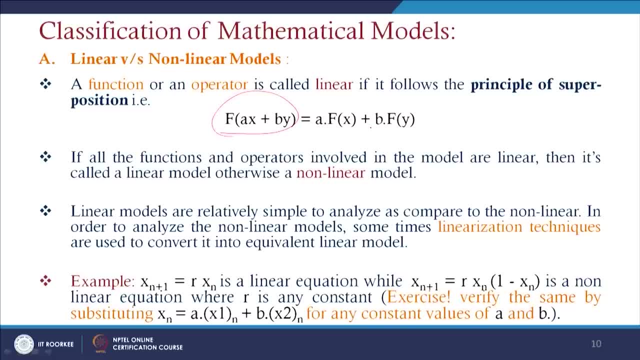 Then it is called a linear model. Otherwise it is a non-linear model. So linear models are relatively simple to analyze as compared to the non-linear. In order to analyze the non-linear models, sometimes linearization techniques are used to convert into a equivalent linear model. 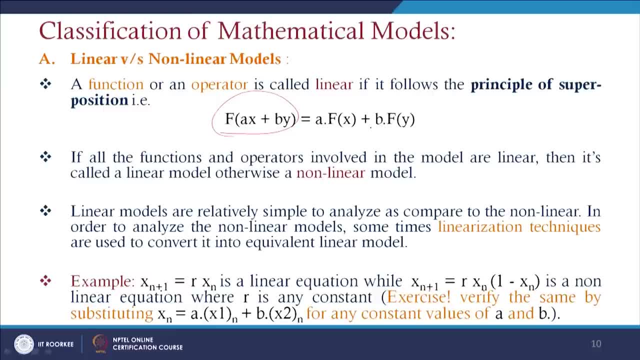 So the popularly known linearization model is Newton's linearization technique. For example, suppose you'll have a equation like: xn plus 1 equals to R of xn is a linear equation, While xn plus 1 equals to R. xn into 1 minus xn is a non-linear equation where R is any. 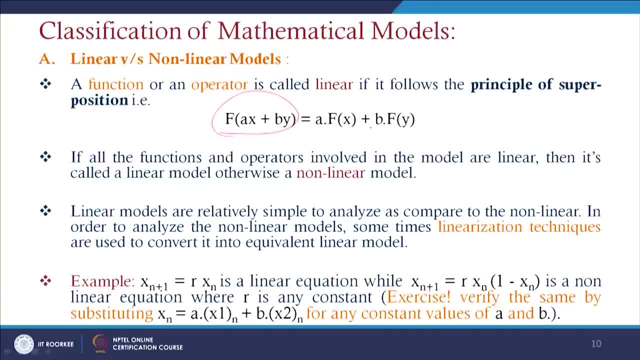 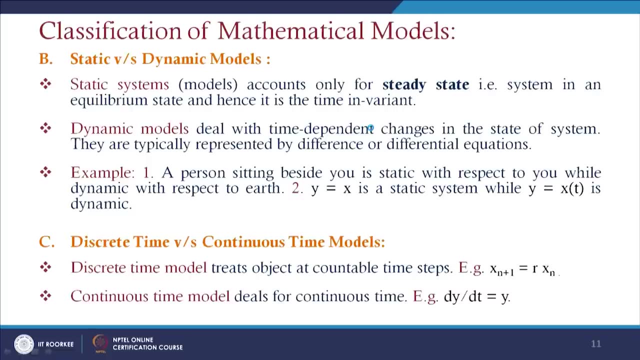 constant. So you can have this exercise. verify the same by substituting xn equals to a into x1 n, plus b into x2 n for any constant values of a and b. So second classification of mathematical model deals with static versus dynamic models. So static systems means it accounts only for a steady state. 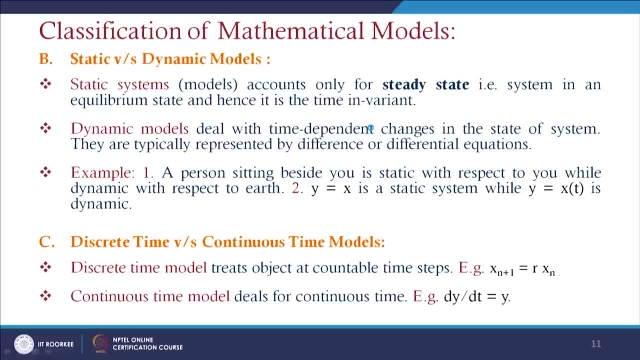 That is, The system is in equilibrium state and it is invariant with respect to time. We can just say the system is in static. Dynamic models means with respect to time, if the state of the system getting changed- they are typically represented by difference or differential equations- is called a dynamic. 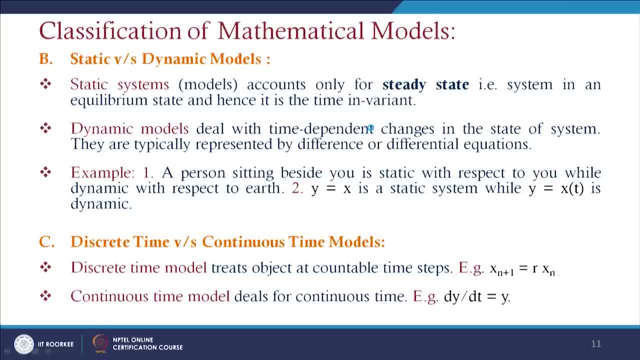 model, For example, if a person is sitting besides you is static with respect to you, while dynamic with respect to earth, suppose, Since earth is rotating with respect to time. Second example: if suppose you are just considering, y equals to x is a static system, while y equals. 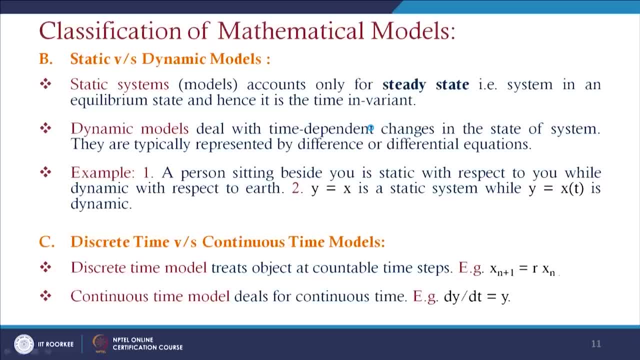 to x of t, where x is a function of time is a dynamic system. So third classification of mathematical model deals with discrete time versus continuous time models. Discrete time model means it we can just treats the object at countable time steps, That is especially: xn plus 1 equals, to suppose, R of xn. 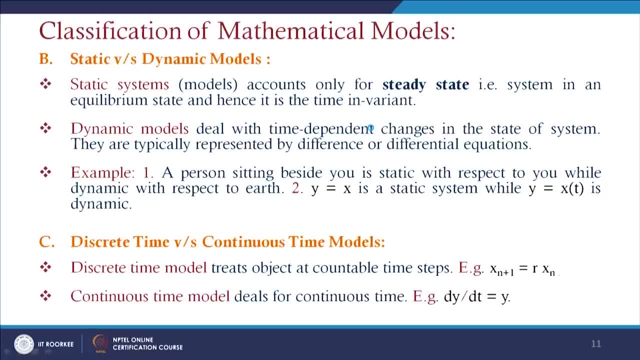 Here And The dynamic model deals for continuous time. that is, dy by dt, this equals to y. If you'll just see this simple differential equation, you can just find that y gets change with respect to t here. So that's why continuously it got change. 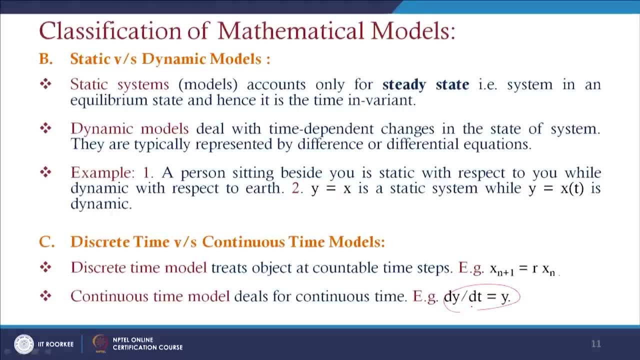 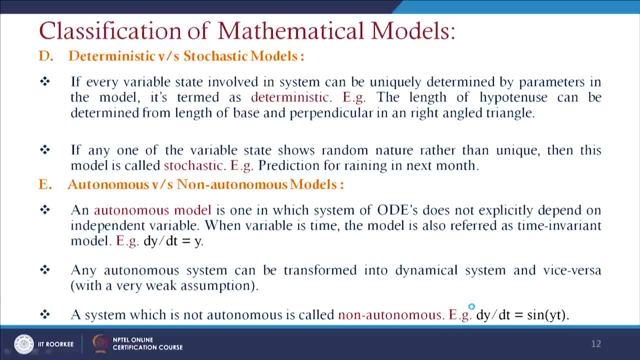 So that's why we are just representing in this sense here. Then we'll just go for like a deterministic and stochastic models. If every variable of the state involved in a system can be uniquely determined by parametric parameters in the model, it is termed as deterministic. 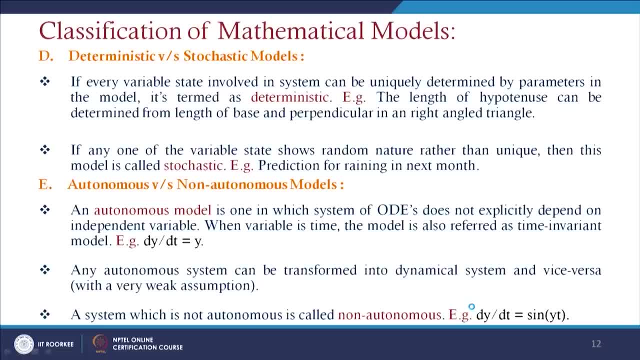 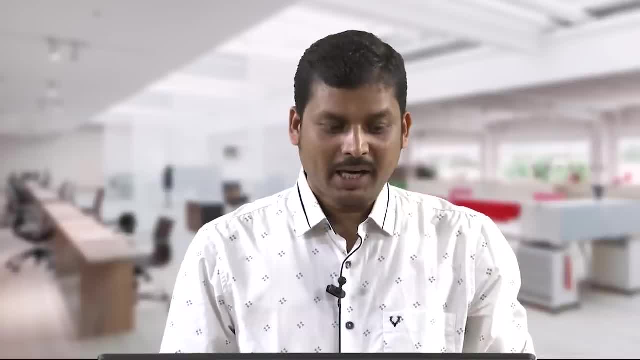 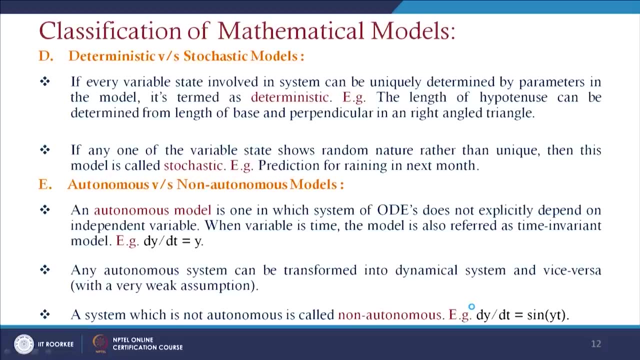 Suppose the length of a hypotenuse can be determined from length of a base and perpendicular in a right angle triangle. Already I have explained this one for this forward modeling And second, stochastic models means if any one of the state variable shows random nature rather than unique, then this model is called stochastic model. 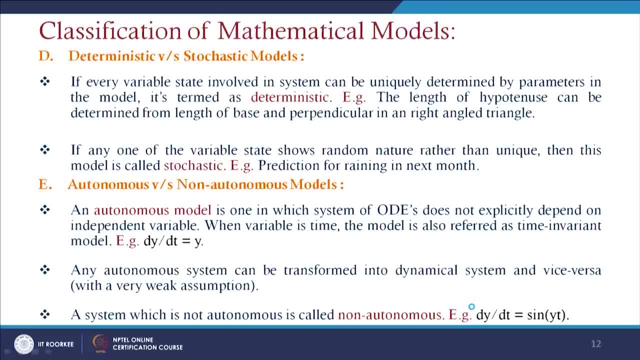 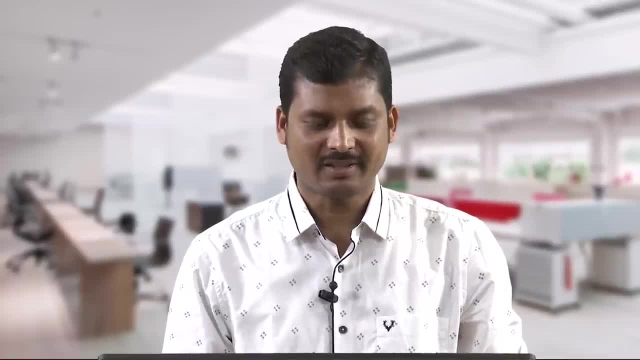 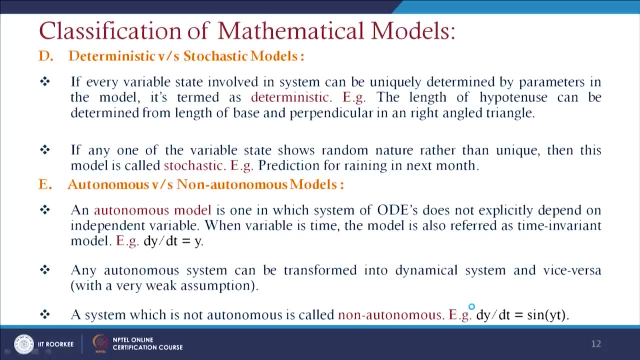 That is especially prediction for raining in next month. So If you'll just like expect the data what it will happen, then we can just say that it is in a stochastic sense And then we'll have like autonomous versus non-autonomous models. An autonomous model is one in which system of ordinary differential equations does not. 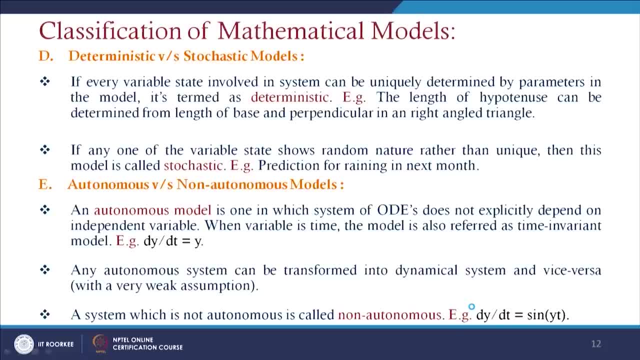 explicitly depend on independent variables. When variable is time, the model is also referred as time invariant model. that is, dy by dt equals to y suppose, And The autonomous system can be transformed into dynamical system and vice versa, with a very weak assumption especially. 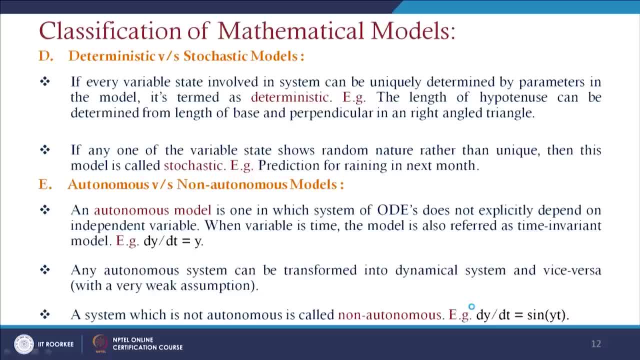 And a system which is not autonomous is called a non-autonomous system. So, especially if you'll just consider this differential equation, that as dy by dt, this equals to sin y of t, suppose. So with respect to time, so both the sides, it got changed so we can just say the system. 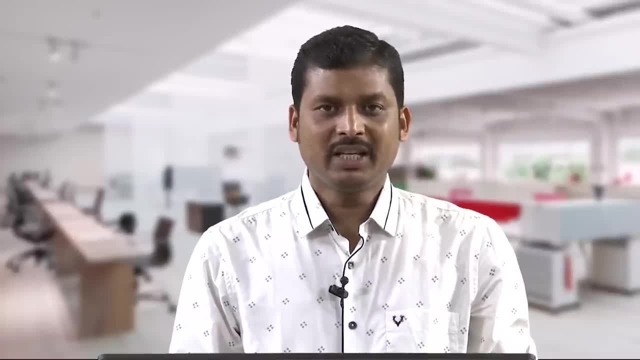 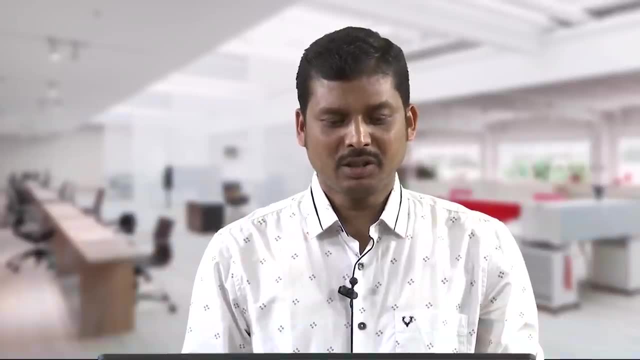 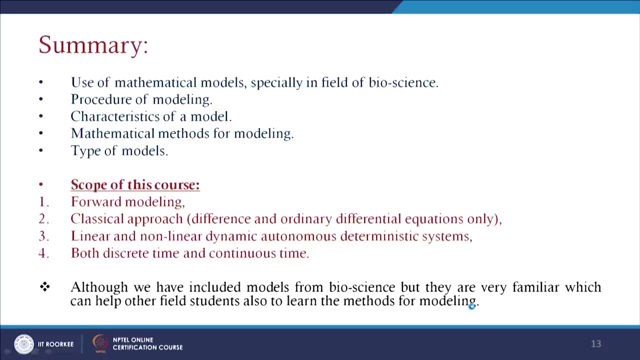 is a non-autonomous there. So, finally, we are just concluding A, Based on this, basic definitions and classifications of mathematical model Here. if we'll just use this- mathematical models in different fields of like engineering or biosciences- we can have a like different models and we first, we can just develop this. 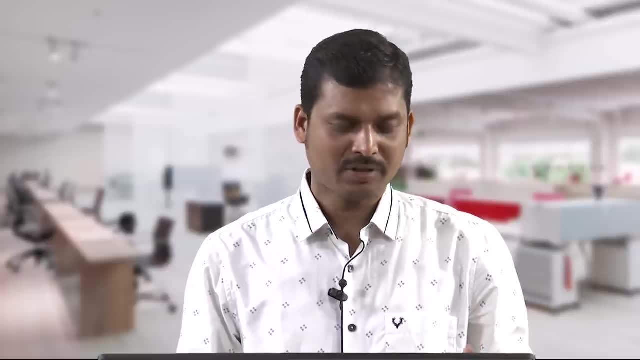 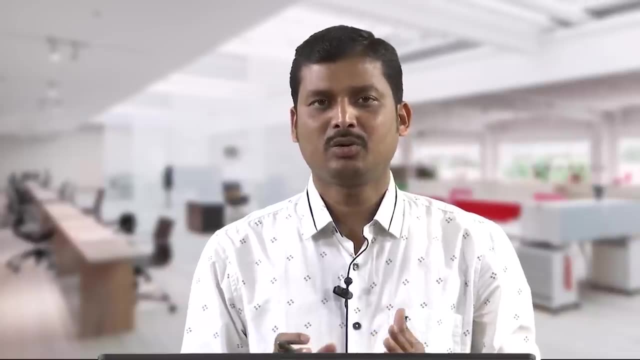 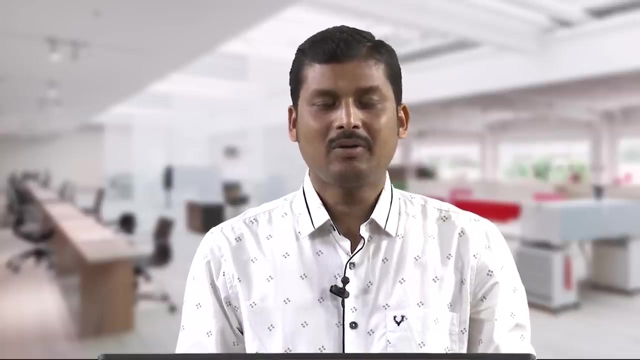 model. then we can just define some of this: approximations with respect to this, variables, and sometimes we can just define this logical operations to combine all this mathematical variables. Then we'll have a proper model. So how we can just formulate a mathematical model, that is procedure of modeling, then characteristics. 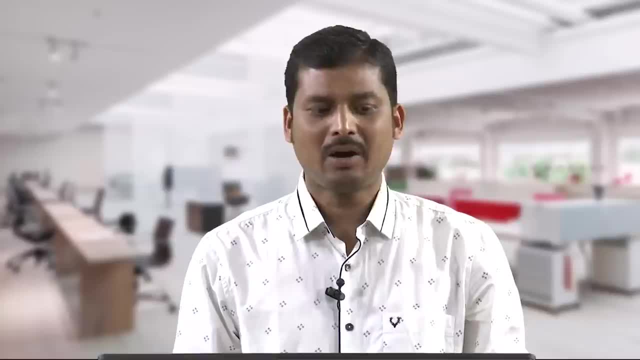 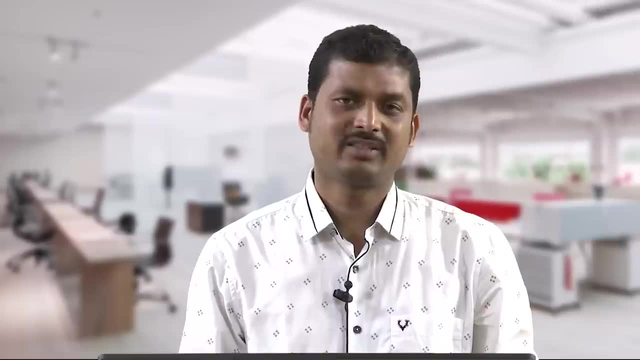 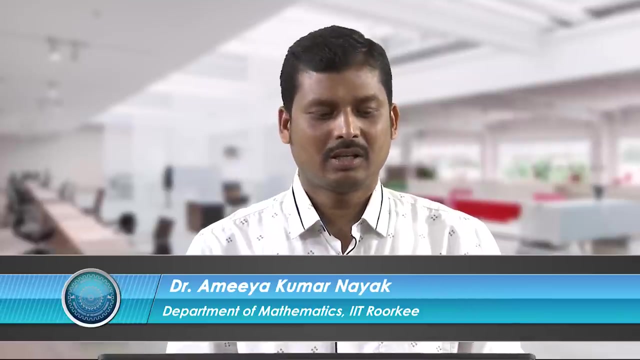 of model. if you will have a mathematical model how we can just find different characteristics or how we can just like predict different characteristics from this model, Then mathematical models for modeling, so different models can be used, and then the type of models, So different class of models we have just discussed till now. 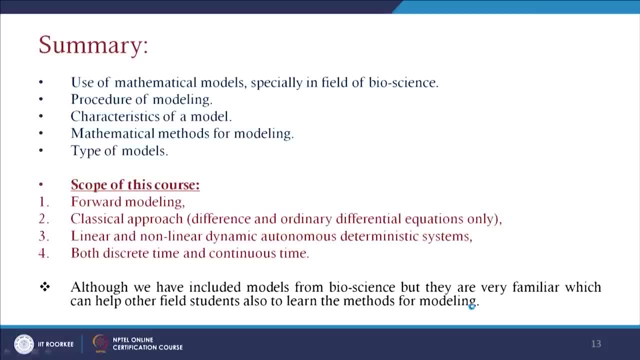 So scope of this lecture, especially forward modeling, classical approach, linear or non-linear, dynamic, autonomous or deterministic systems. both this discrete time and continuous time can be used for the mathematical modeling, Although we have included models from bioscience, but they are very familiar, which can help.